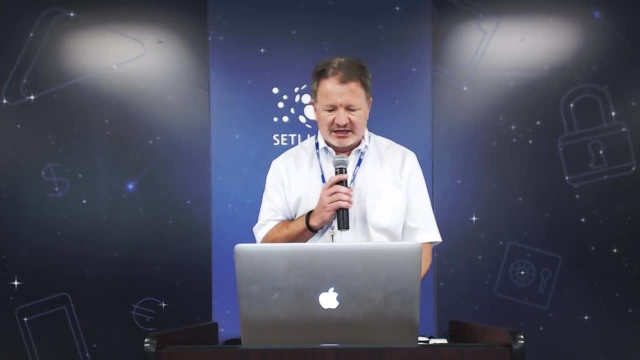 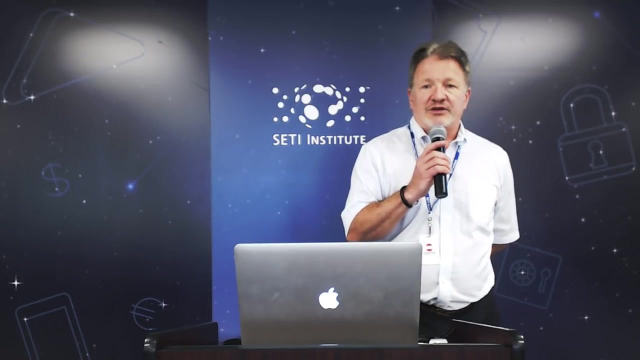 Dr Bruce McIntosh from Stanford University. He will be speaking to us. His presentation is called the direct imaging of extrasolar planets and the Gemini planet imager, of which he and his colleagues are pioneers in new instrumentation that is allowed to be used. 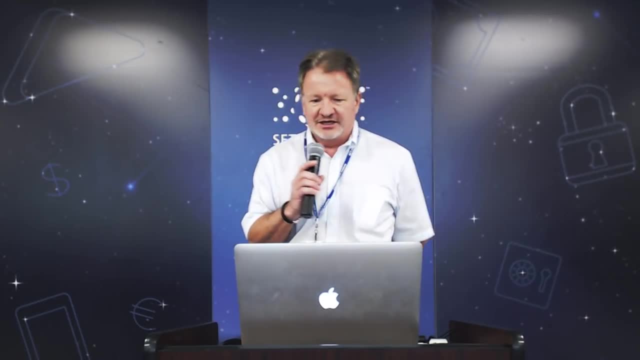 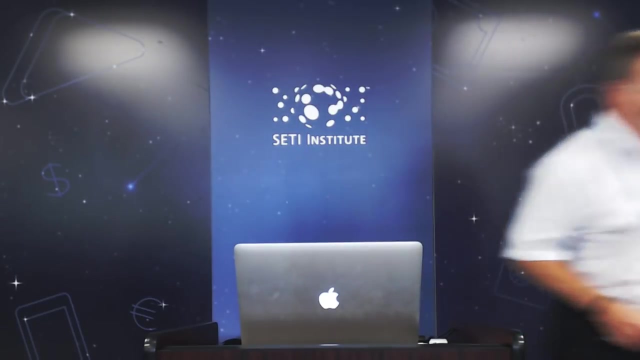 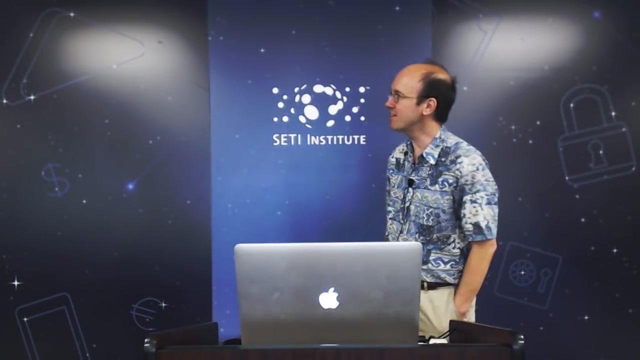 Dr Bruce McIntosh from Stanford University. He will be speaking to us. His presentation is called the direct imaging of extrasolar planets and the Gemini planet imager, of which he and his colleagues are pioneers in new instrumentation that is allowed to be used. 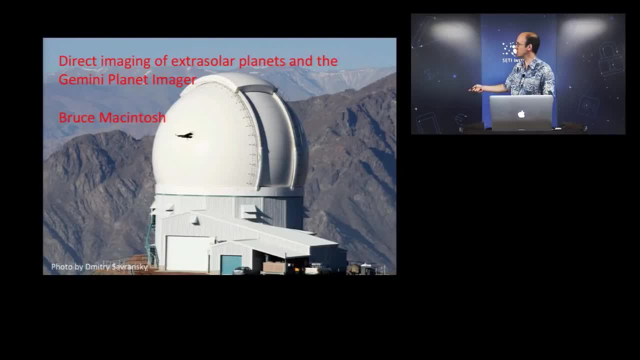 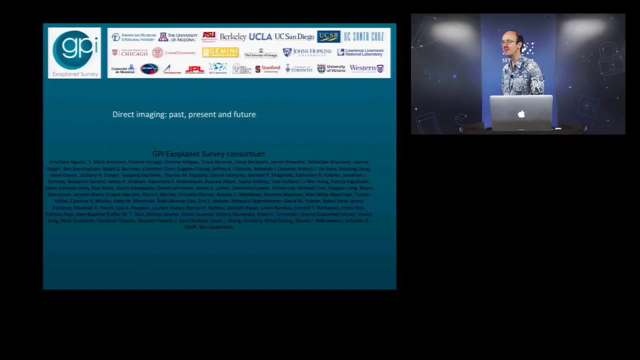 Dr Bruce McIntosh from Stanford University. He will be speaking to us. His presentation is called the direct imaging of extrasolar planets and the Gemini planet imager, of which he and his colleagues are pioneers in new instrumentation that is allowed to be used. 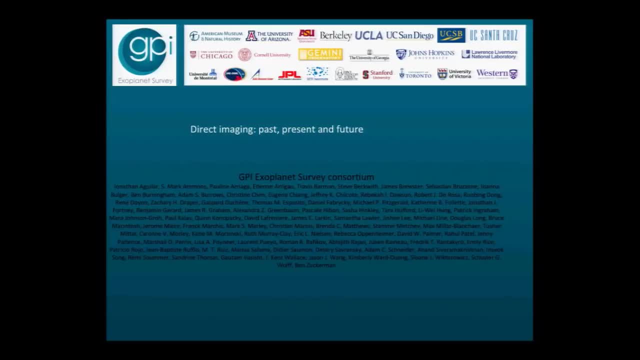 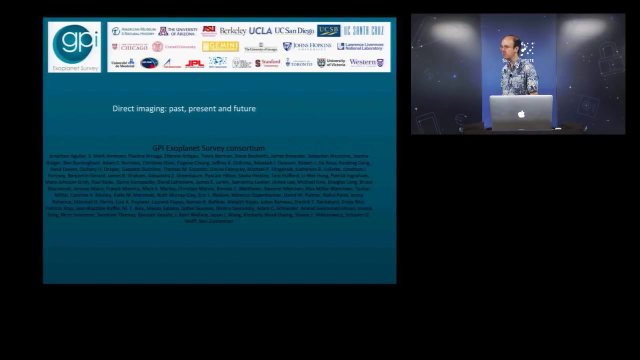 Dr Bruce McIntosh from Stanford University. He will be speaking to us. His presentation is called the direct imaging of extrasolar planets and the Gemini planet imager, of which he and his colleagues are pioneers in new instrumentation that is allowed to be used. 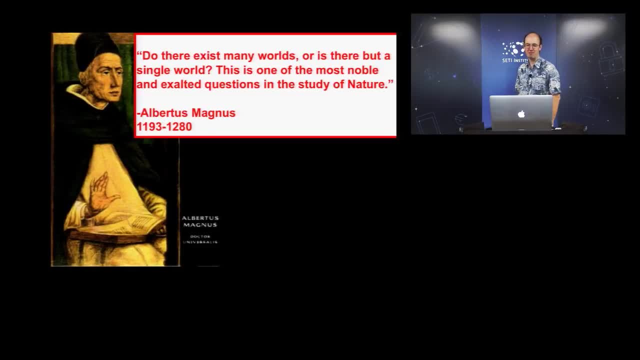 Dr Bruce McIntosh from Stanford University. He will be speaking to us. His presentation is called the direct imaging of extrasolar planets and the Gemini planet imager, of which he and his colleagues are pioneers in new instrumentation that is allowed to be used. 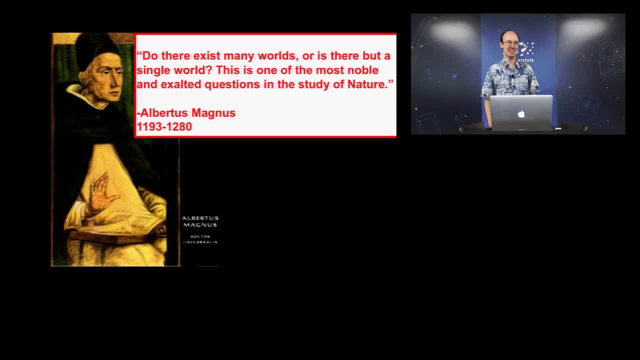 Dr Bruce McIntosh from Stanford University. He will be speaking to us. His presentation is called the direct imaging of extrasolar planets and the Gemini planet imager, of which he and his colleagues are pioneers in new instrumentation that is allowed to be used. 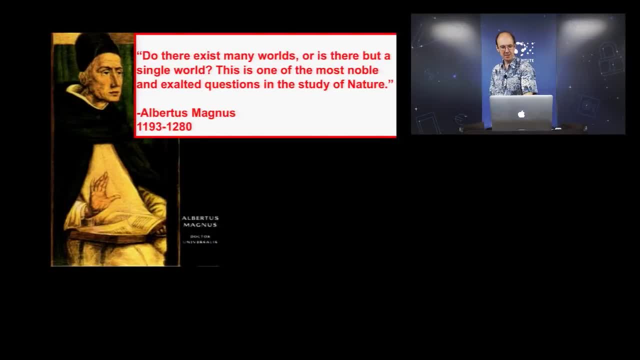 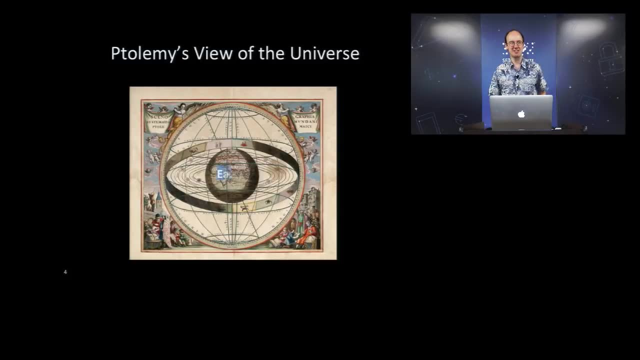 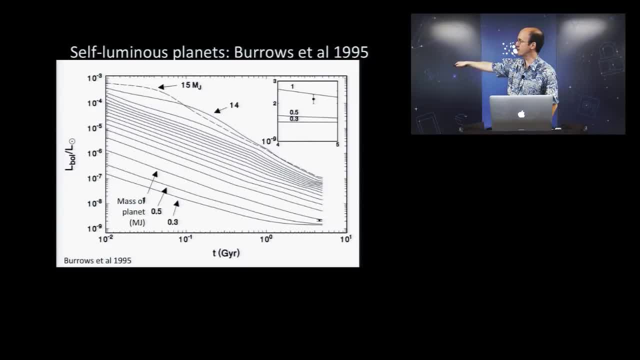 TheDентcom, theDентcom, theDentcom, theDENTcom, HetheDevel campus- and dimmer as they cool down. And if you catch them at 10 million year old ages, the planets are bright enough, so they're only 10,000 times. 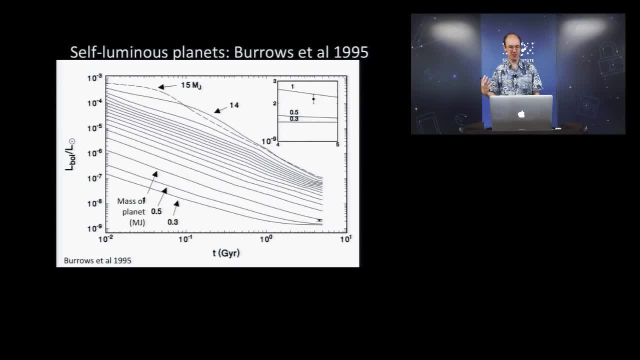 or a million times fainter than their star, which is still pretty faint, but a lot better than a billion that Jupiter is sitting at way down here right now. So, by looking for planets that are young, which we can do by looking at stars that are young, 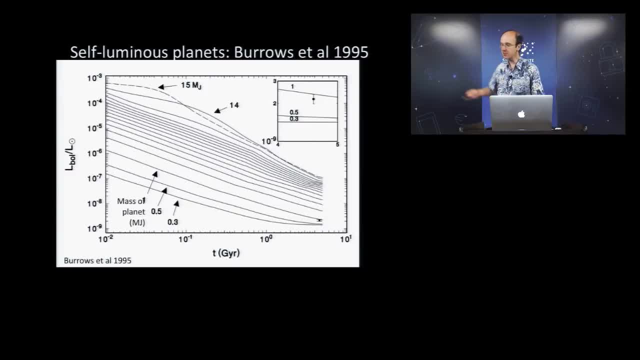 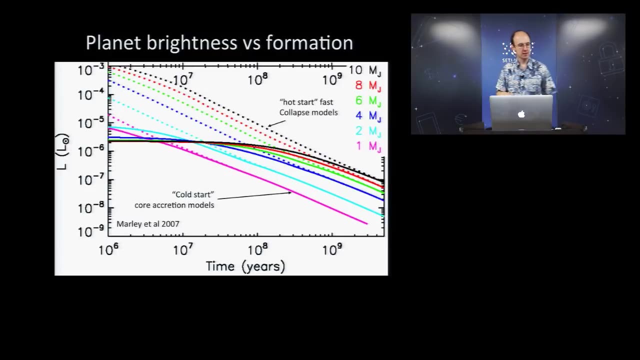 the planets are potentially detectable. A complication in this is that this is another one of those sort of pre-Copernican graphs where people put it together assuming a simple process of planet formation. A more sophisticated approach to this accounts for the two different models of planet formation. 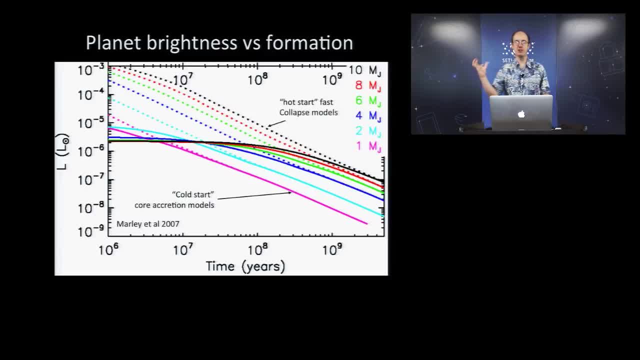 that I talked about And in particular, if a planet forms through the core accretion process, form the core first, suck all the gas in, like we think our solar system formed. that releases a lot of the planet's energy early on. 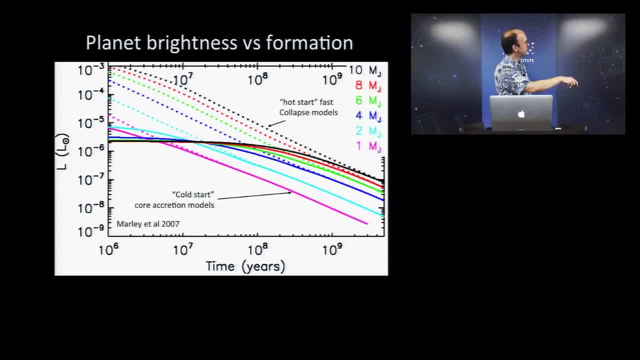 and later on the planet is dim. So one last version of this graph. This here color code, show each different size of planets: medium-sized Jupiter-sized planet. really big 10 Jupiter mass planet. If they form through the fast collapse process, then they're really, really, really bright. 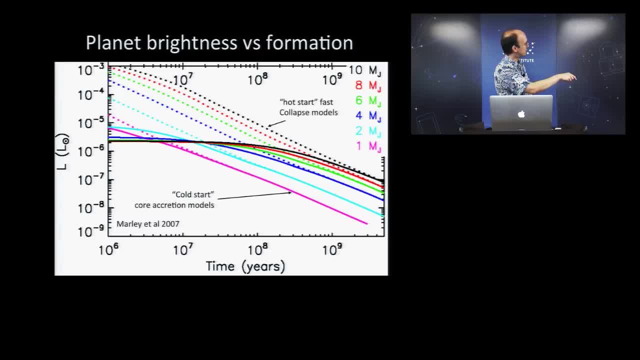 when they're young and gradually cool down. If they form, on the other hand, through the core accretion process, like we think our solar system did, they actually never are very bright early on. They kind of sit there percolating away. 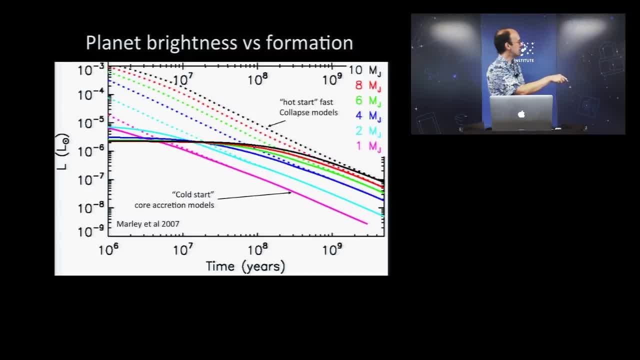 and then gradually rejoin the cooling tracks of the other planets. So it actually is a sort of mixed blessing. On the one side it means where we're sensitive with our early equipment to sort of 10 to the minus 5, 10 million times fader than the sun. 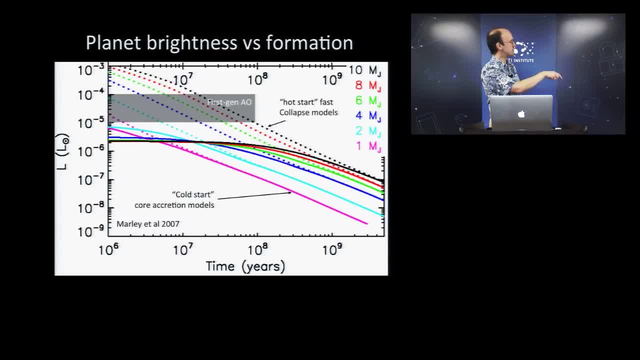 we can only see planets if they start out hot. But someday, if we could see both kinds of planets, maybe we could tell which way they form by looking at how bright they are versus time. So a bunch of groups searched, using first generation adaptive optics system for planets like this. 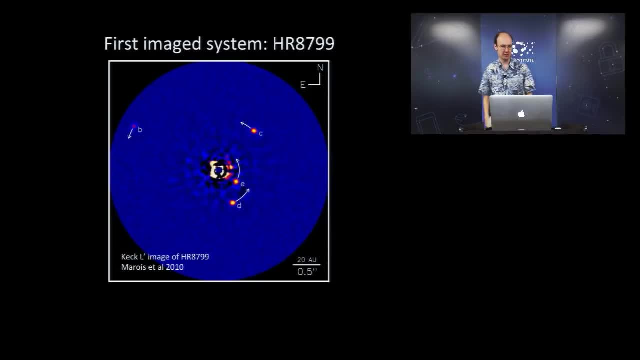 This is one example of a success- probably the most spectacular example- using that, the HRD790.. The HRD790 system that Christian Marois and a number of people, including myself, found in 2008 and 2010.. So these are actual pictures of planets. 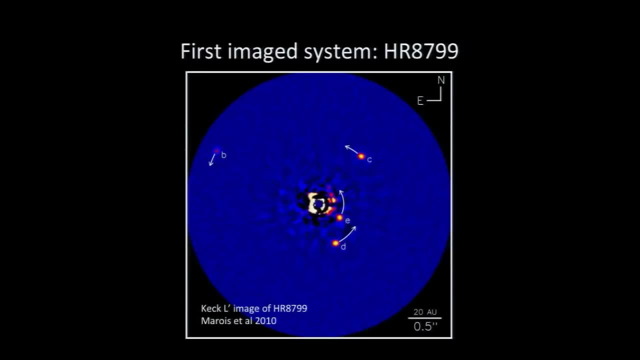 What you're seeing here is the star kind of behind a mask. A lot of image processing has gone into it, but a little bit of leftover starlight are these white blobs here and these black blobs here? But the dots are actual infrared radiation from four planets. 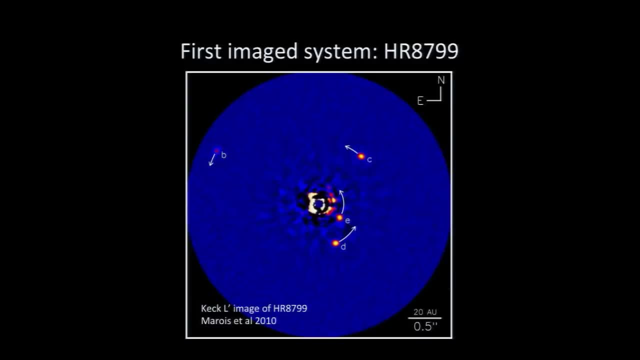 The arrows are not giant arrows that were drawn on the sky. They're there to guide your eye in the process. The star is about 50% more massive than our sun. The planets are about five to seven times the mass of Jupiter, So they're big planets about 1,000 degree temperature. 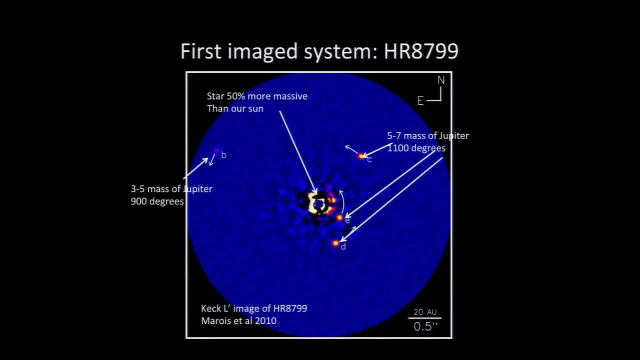 for the outermost ones, maybe 900 degrees Kelvin for the innermost ones, But they're real. So we can actually now look at a whole other solar system from outside and see its individual planets and see them moving around. In some ways, this whole other solar system. 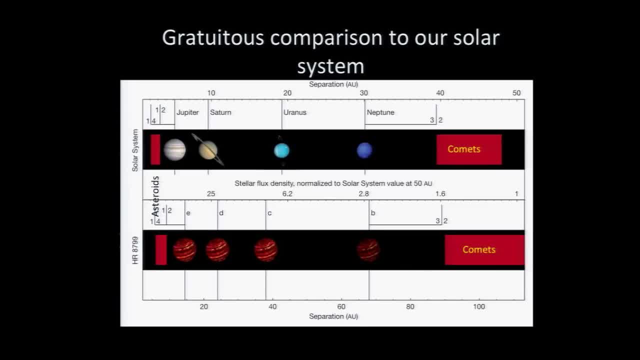 is kind of like our solar system. We have four giant planets. It has four giant planets. Our solar system has a belt of asteroids and a belt of comets- the Kuiper belt. There's evidence from infrared observations. this solar system also has a belt of asteroids and a belt of comets. 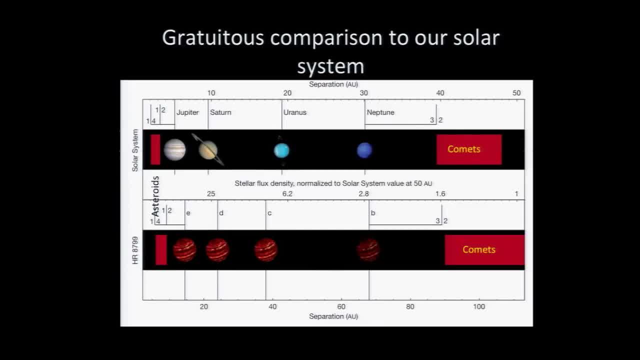 at large angles and that there's a gap between those right where the planets are, which makes sense because the planets would clear out asteroids and comets there, just like they do in our solar system. Otherwise, it's not like our solar system. 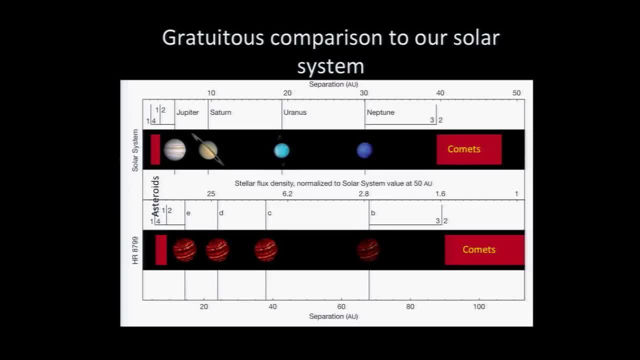 The total mass of these planets is probably 30 times the total mass of planets in our solar system. Their orbits are bigger, but of course it's a bigger star, So it kind of makes sense that that's going on And we can watch them orbit. 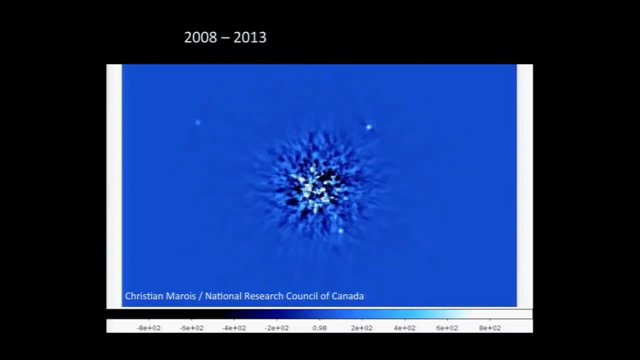 This is just an animation Christiane Merouat put together of data going back to their discovery in 2008.. So some 2013 or so epochs. The innermost planet is hard to see. You can only see it when the weather is really good. 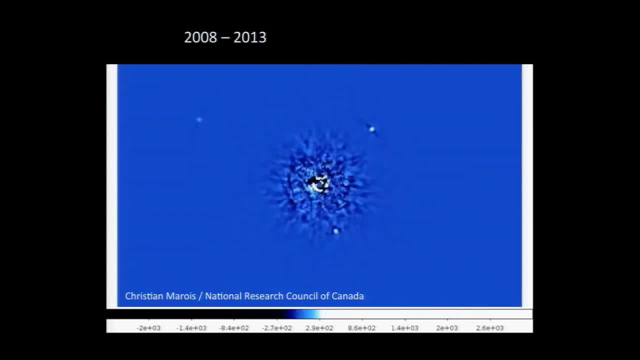 So it's not in all these blobs, But there's the other three. They're moving. They're moving like Kepler's laws say they should move. So this one is going really slowly because it's far from the star. This one is going quite fast because it's. 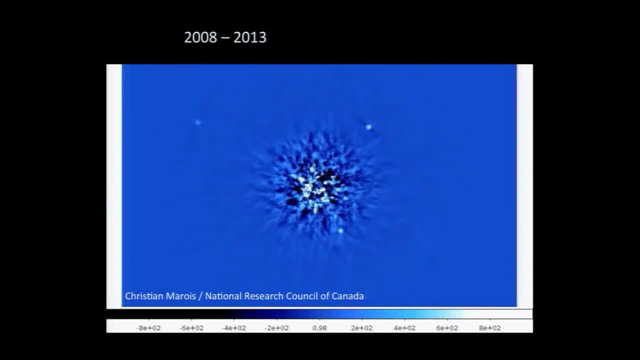 close to their star. It's not a surprise. Kepler's laws, of course, are Newton's laws. They apply everywhere in the universe. But the fact that we can see Kepler's laws from outside, that we can see a whole solar system going around the way, 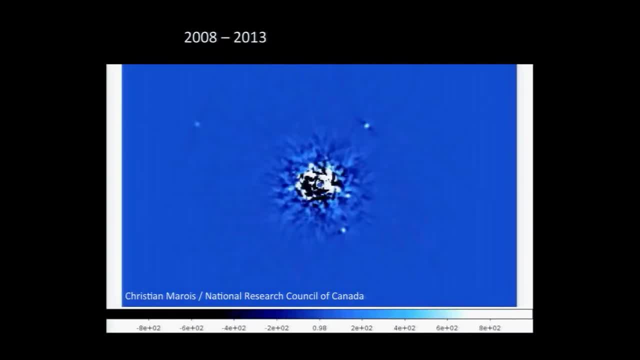 once upon a time we would have just had animations like the one I showed you earlier that we can see in real data. real life is actually pretty amazing. So I said, why we might want to directly image these planets is to think about their composition, what 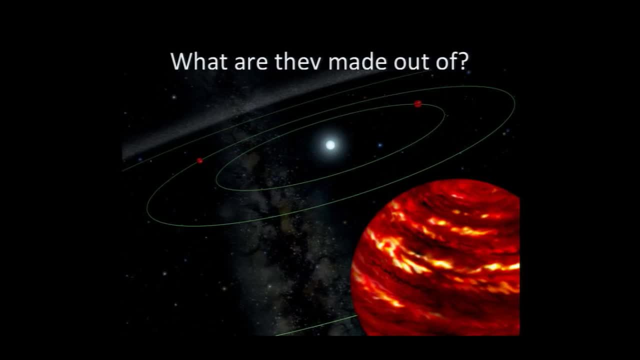 they're made out of. We had our press release figure too, And I'll show one for if you want to hear it on the left. But of course we don't see that, We just see the dot of the planet. But because we can image it, we can actually say something more. 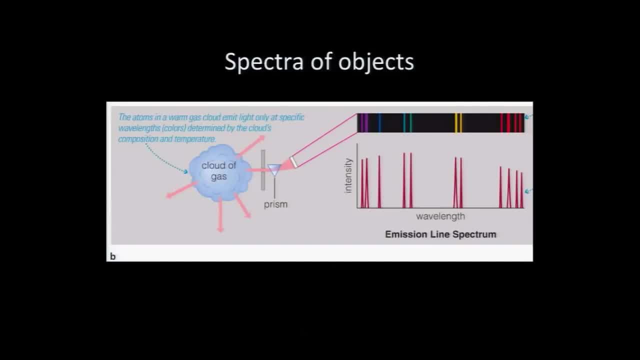 about its composition. So I'll just remind people a little about spectroscopy. Every element in the universe has a distinctive footprint of light that it gives off. The atoms that compose it have certain light levels of energy they like to absorb or emit, And so it will only give off certain particular colors. 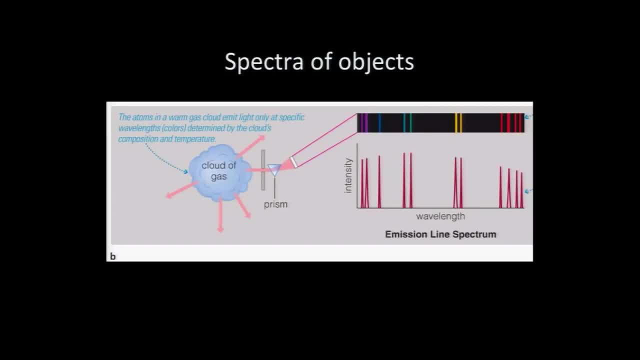 of light And you've all seen this in your high school physics experiments or college physics experiments. If I have a cloud of hot gas and I feed the light from it through a prism, I'll get a particular distinctive chemical fingerprint, And that chemical fingerprint differs. 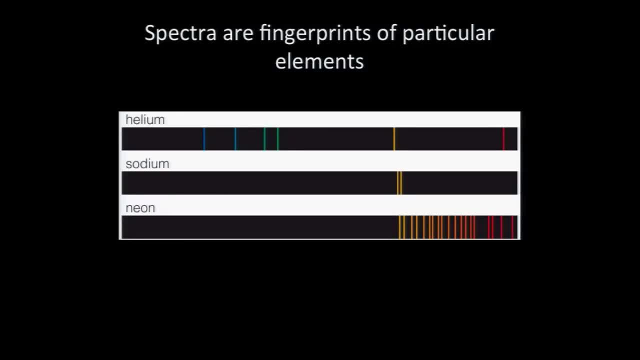 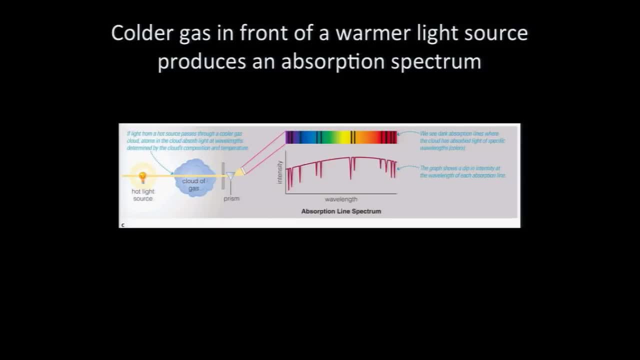 for different elements: helium, sodium, neon, et cetera. If you're a scientist, rather than looking at these color bars, you might choose to make a plot, a graph of the intensity of light versus wavelength If you have a hot light source behind a cold cloud of gas. 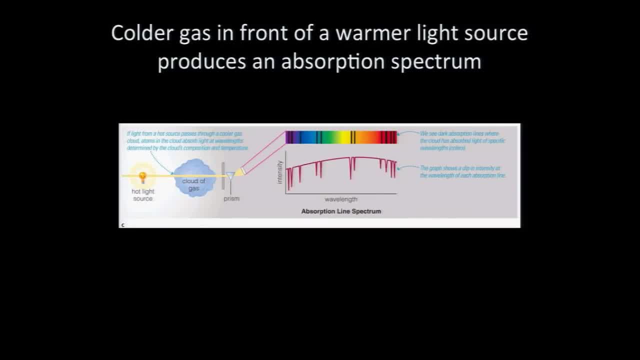 instead of seeing bright lines, you see dark lines, where this cloud of gas likes to absorb certain particular wavelengths. And if I plot the intensity of light versus wavelength, you can see the dips as the intensity goes down again due to the chemical fingerprints. 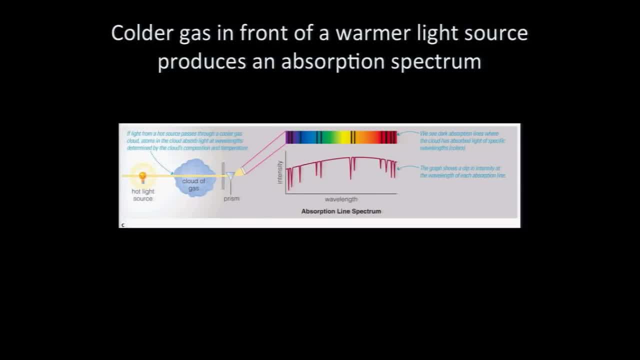 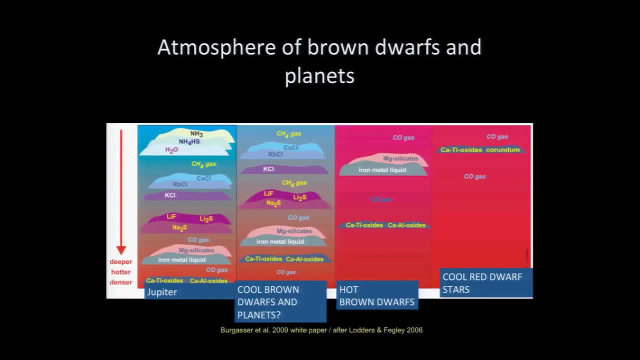 And so, in turn, if I can get light from my planets, I can start to say something about the chemistry of their atmosphere. We thought their chemistry would look a little bit like this, So these are just stylized cartoons of the atmospheres of various objects. 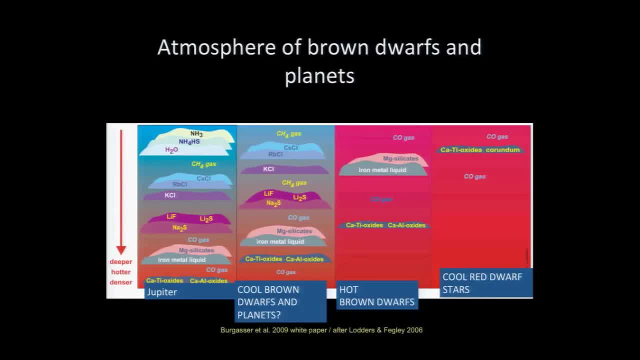 From right to left. the coldest stars have atmospheres that are mostly gas, but have actually clouds of materials that are solid at high temperatures, like titanium oxide, The brown dwarfs, especially the hotter brown dwarfs. those clouds live deeper inside the planet. 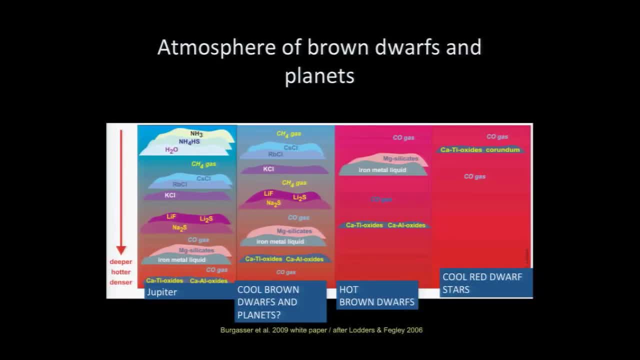 Lighter weight clouds are higher up and their atmosphere is full of carbon monoxide, which you could see in a spectrum- The cooler brown dwarfs- and we thought planets would look like cooler brown dwarfs. the clouds are even deeper in their interior. 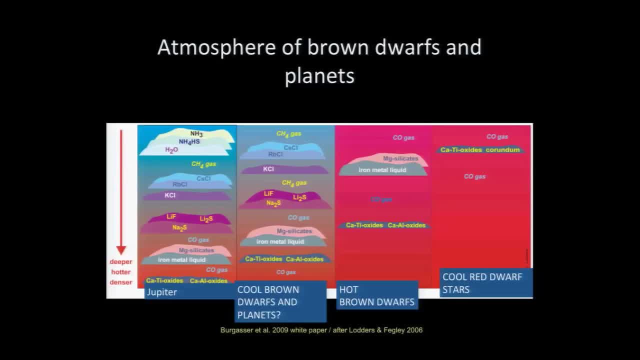 Up at the top, where the atmosphere is cool, you can get compounds like methane, And so we thought we would see radiation coming up from the hot clouds through the methane and we'd see the spectral fingerprints, the absorption lines of elements like methane. 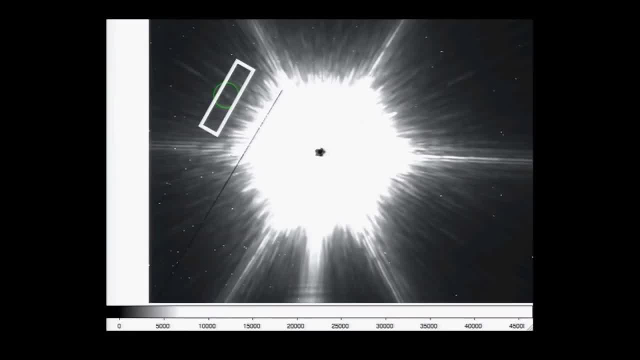 when we looked at our planets, So we decided to look for this. Here's a Keck image, without a lot of image processing now, showing what one of the planets looks like relative to the very bright star, And this is the field of view of the spectrograph we used for it. 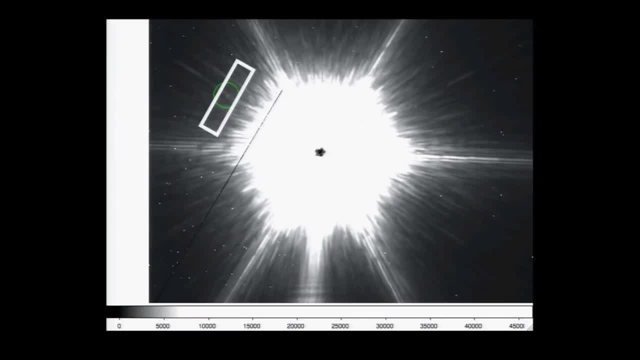 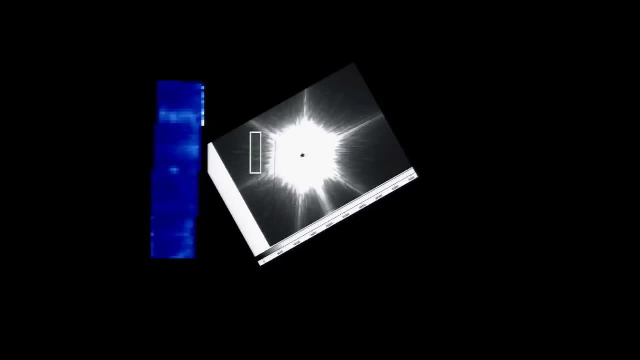 The spectrograph. the instrument called OSIRIS is a very special spectrograph. It doesn't just measure the spectrum of one object at a time. Instead it takes a three-dimensional picture where for every pixel in the image I actually get a little microspectrum. 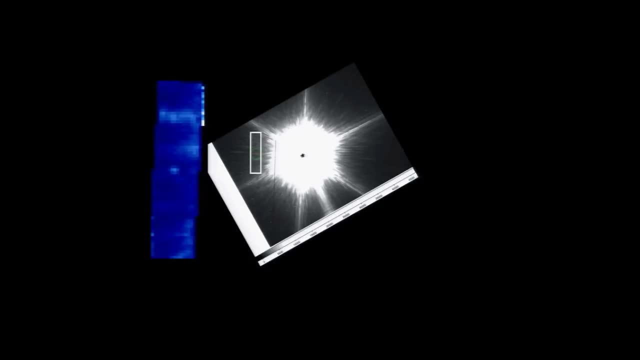 I get the intensity as a function of wavelength, So I can measure the spectrum of every object it looks at all at once over a small postage stamp field of view, And I can show that by animating this. Here's the total image, with a little dot there that 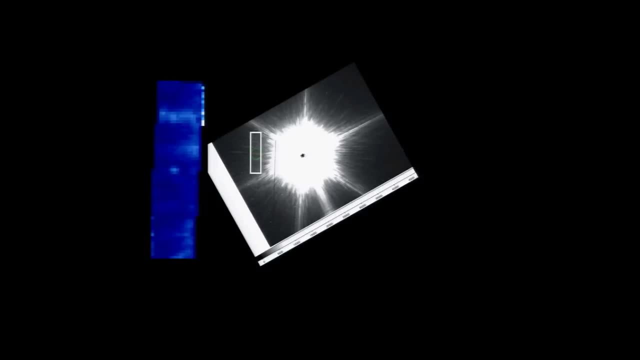 turns out to be the planet. All the streaks you're seeing in this image are scattered light diffraction and optical interference off the Keck telescope. Because they're a process made by diffraction, each of these little streaks- actually different wavelengths of light- go to different positions. 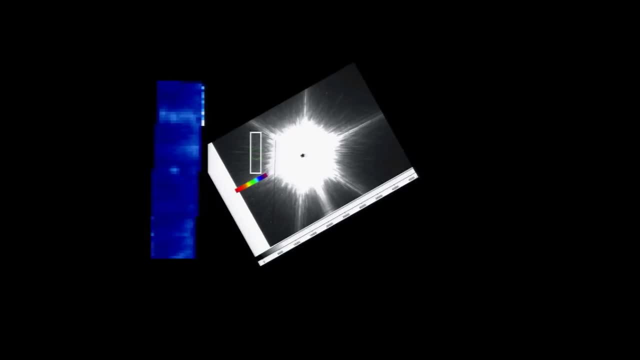 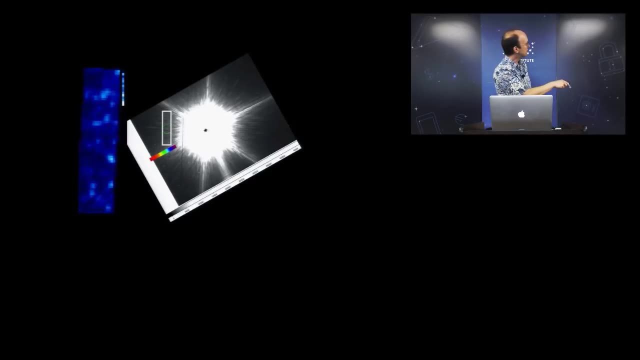 in it. These are like tiny little extended spectra where red light scatters far away from the star and blue light scatters close. I can turn on an animation where I'm now stepping from long to short wavelengths And all of the artifacts, all of the scattered light. 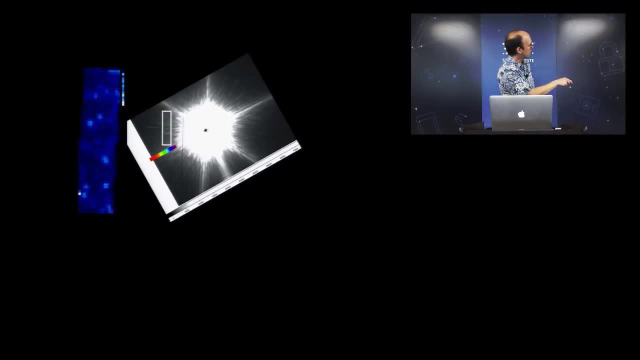 have positions that change as you go from short wavelength out to long wavelength, short wavelength out to long wavelength. The planet always stays at the same position at all wavelengths, And so you can use that to get rid of all the scattered light and say, yeah, there's the planet. 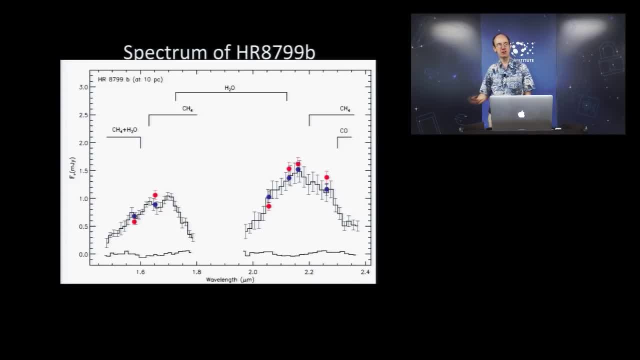 Stack it up, And so we extract that, We do some math, We turn it into a quantitative plot of intensity versus wavelength: intensity, wavelength, And you can see in this this is near infrared radiation, because that's where the planet's bright. 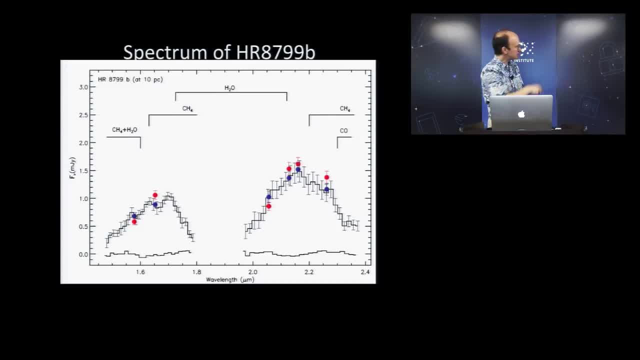 So long wave visible light would be somewhere off here. long wavelengths of light. You can see some chemical fingerprints. for example, carbon monoxide absorbs very strongly here Water. this is absorption due to water vapor in the middle. We don't actually make a big deal about water vapor. 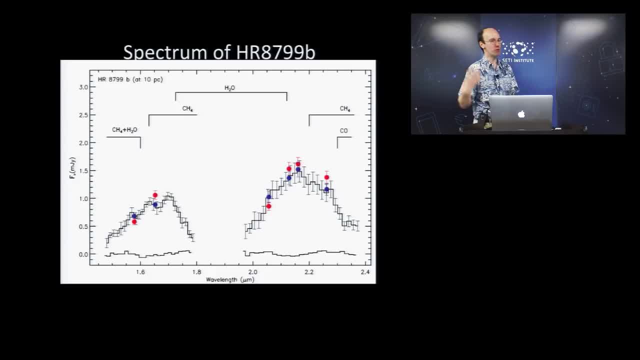 because it's hydrogen oxide is the most common thing in the universe. Of course there's water- It'd be weird if there wasn't- But there's a huge water vapor absorption signature present there. What there's not is methane is supposed to make a big absorption signature here. 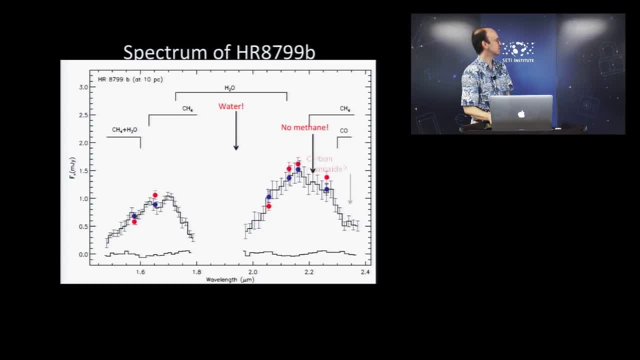 and it didn't show up. So we see the water. We don't see any methane, We see carbon monoxide And the overall radiation we see we think is from hot, thick clouds of liquid metal. So it's confusing that we were seeing these thick clouds. 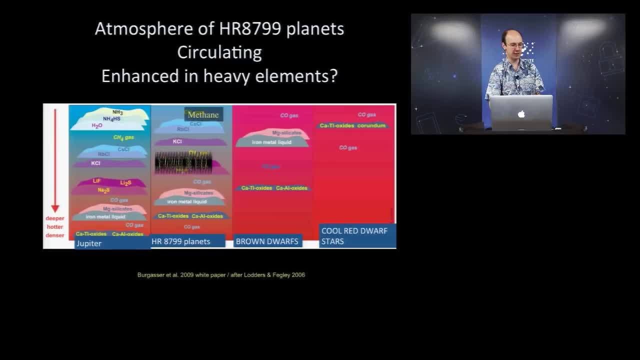 and not seeing the methane. What we think is happening is that the planet's atmosphere circulates, pulling up the clouds to the top of the atmosphere, where we can see them, the clouds of liquid metal, and pushing down the methane where it gets destroyed. 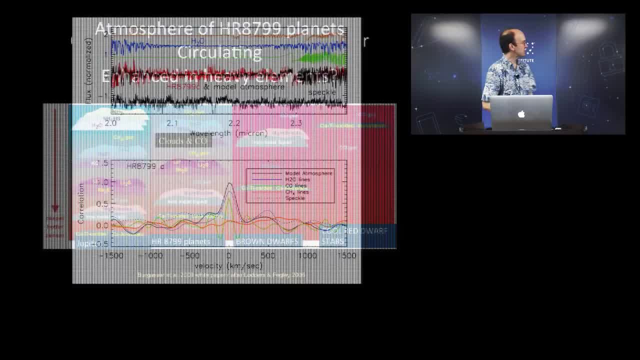 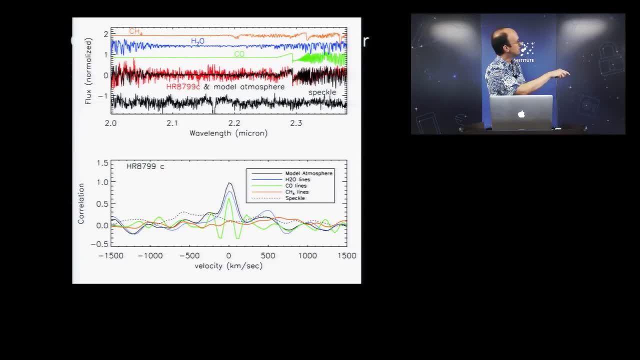 in the inside of the planet Because we can study its light. we can actually study it at very high levels of detail. Here's a zoom in on a different version of that spectrum. Here's the real data And each individual little wiggle in this. 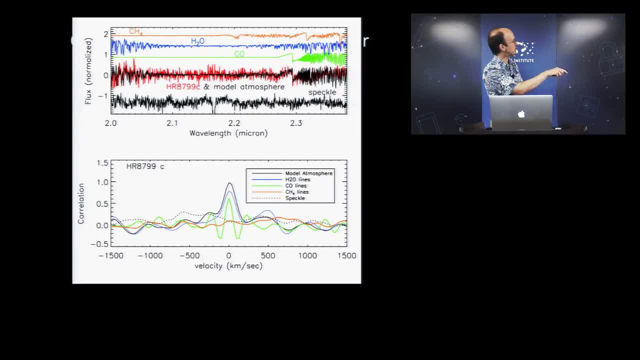 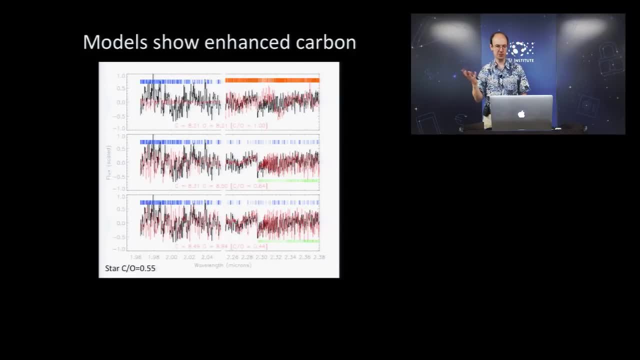 especially out here, actually corresponds to a real feature from the spectrum, especially of water and carbon monoxide, but not of methane. We can use those models- I won't go through this in detail, but to measure those things like the ratios of carbon. 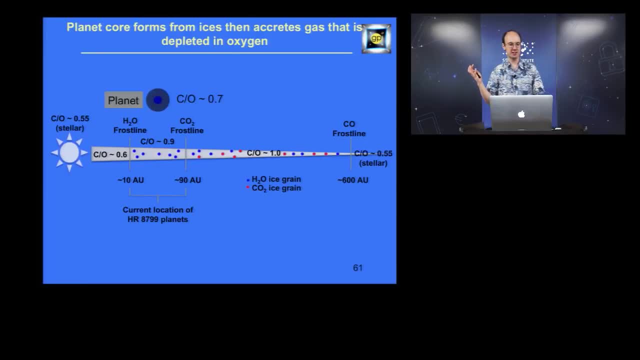 to oxygen in it And we find that the planet is somewhat enhanced in heavy stuff, carbon and oxygen compared to hydrogen in a way that says maybe it did form through the core accretion process, like Jupiter did in our solar system. That was interesting. 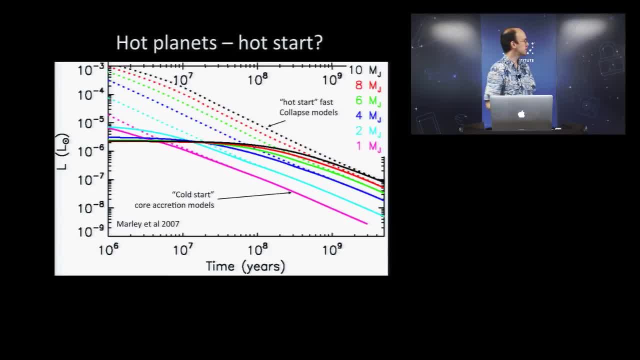 On the other hand, the planet is way too bright to have formed through that process. Back to this graph: brightness of planet versus age. the planets that form through the fast collapse process, the dotted lines, the planets that form the old-fashioned core way, like our solar system. 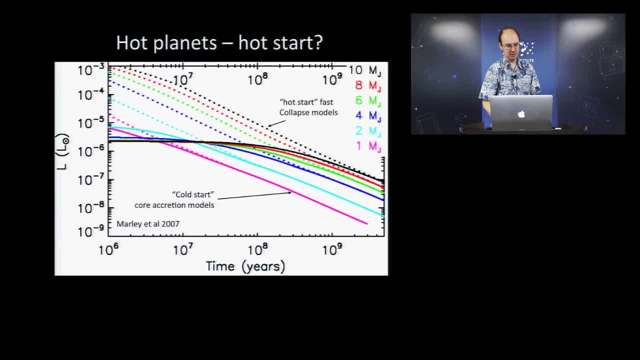 the solid lines. different colors meaning different masses of planets. The HRD 799 planets kind of live here. They're maybe 20,, 30 million years old. They're only 10 to the minus 5 times the brightness of the star. 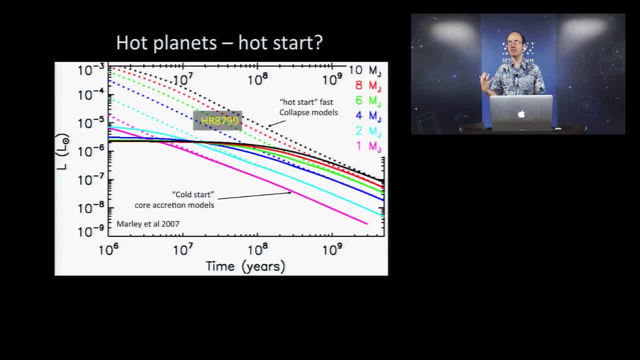 And so it's really hard to make those through a core accretion process. They're too bright to form the way we think Jupiter did, But their chemistry says they form the way we think Jupiter did, So there's actually a lot of confusion. 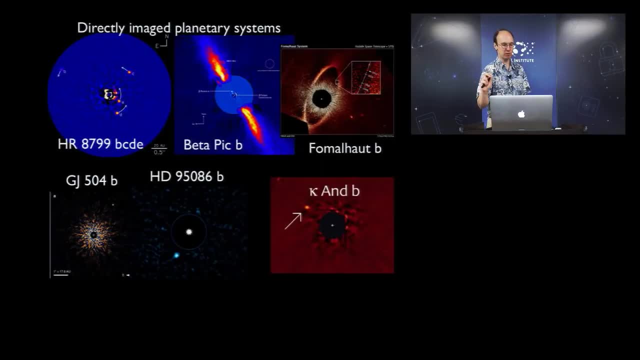 about how you could form these planets And, in fact, although there are a lot of directly-imaged planets, there's no clear consensus. Here's some other ones, like Beta Pictoris, which is in the middle of a beautiful disk of dust. 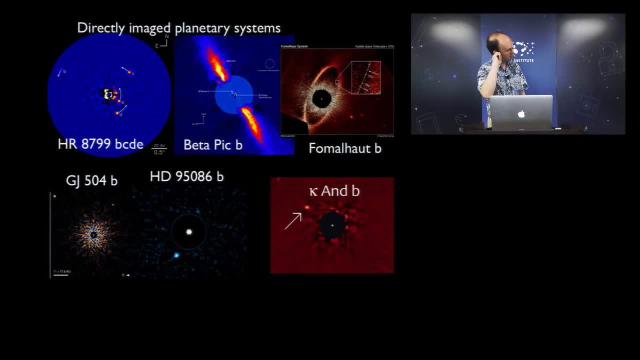 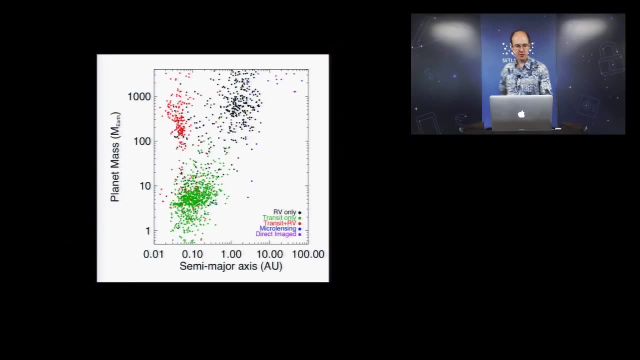 a couple of others with serial numbers. There's no clear consensus on how these directly-imaged planets could have formed and no evidence yet that they formed the way our solar system did. Showing this again: number of planets versus semi-major axes, all the Kepler discoveries. 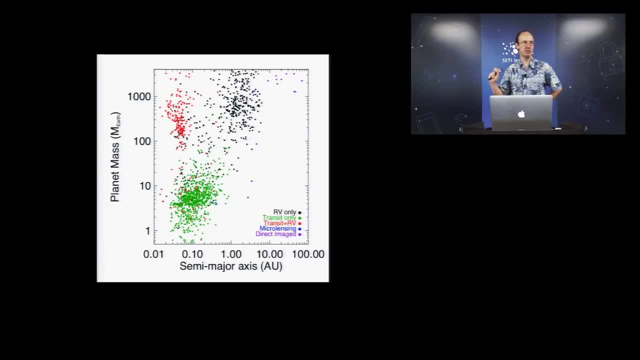 all the Doppler discoveries. if you're a direct imaging person and you show this graph a lot, it actually makes you a little bit sad, because of course there's 1,000 Kepler planets. There's only a handful of directly-imaged planets. 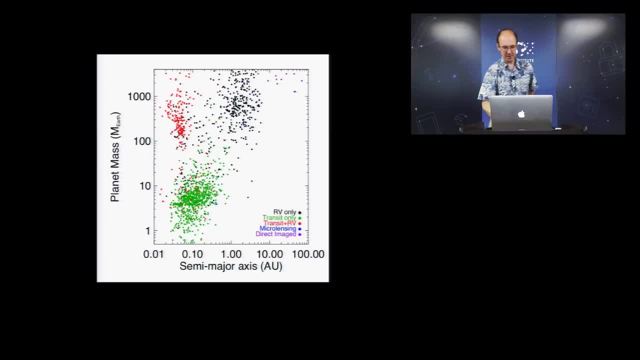 But some people's reaction is not to get sad but to figure out how to do better. First, one thing that's interesting to do is show only the planets that we actually do have spectra of. It turns out for transiting planets, like Kepler finds for a handful of cases. 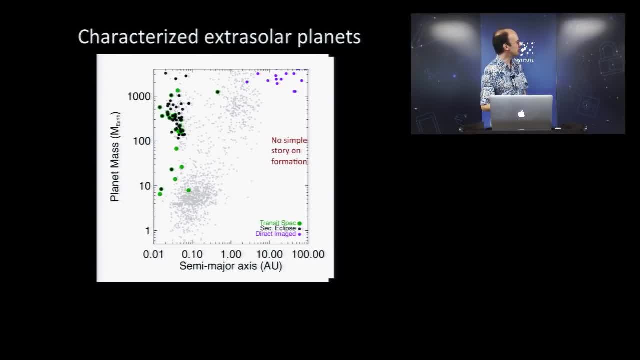 you can also measure their spectra. It's a separate talk that I'm sure you've had people do, I won't go into it. But every direct imaging planet you can also do it, And so direct imaging, Direct imaging is a large fraction of the planets. 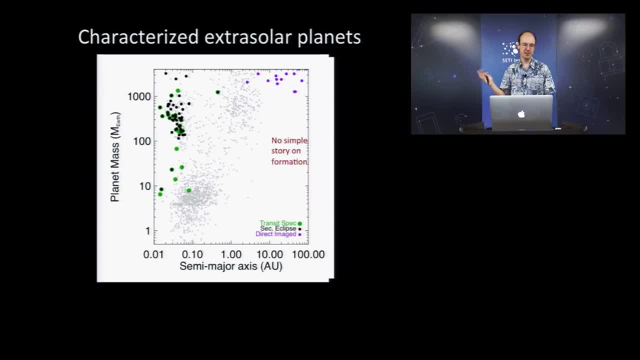 that we've ever actually even gotten close to measuring their composition of, And so that makes us feel better. But really we'd like to find- if not 1,000, like Kepler, which we're never going to do- enough more planets. 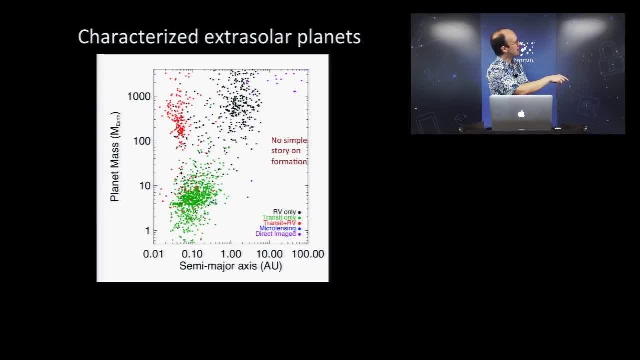 to fill in this direct imaging region and also to bridge this gap. The farthest out we can see with Doppler techniques versus the closest we can see with direct imaging. Direct imaging: it's easy to see planets when they're far from the star. 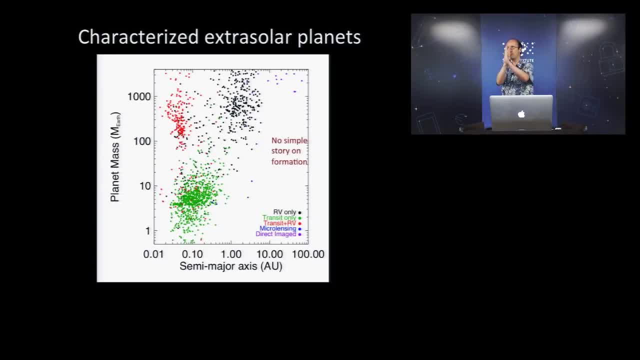 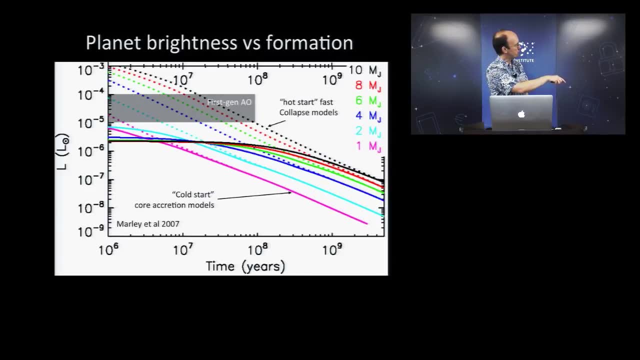 Doppler. it's easy to see them when they're close to the star. We haven't quite reached the point where those overlap, but it would be enormously powerful if it did. And finally, if we want to see more planets and maybe see the ones that formed in the cold way. 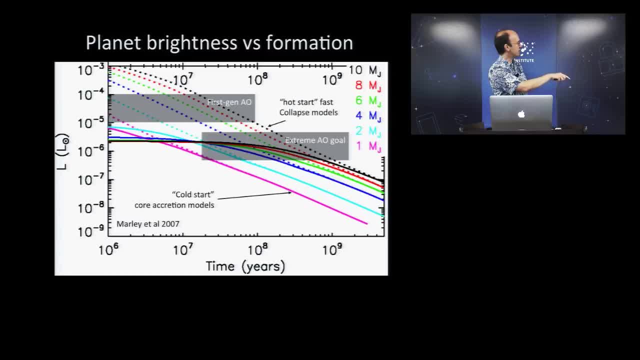 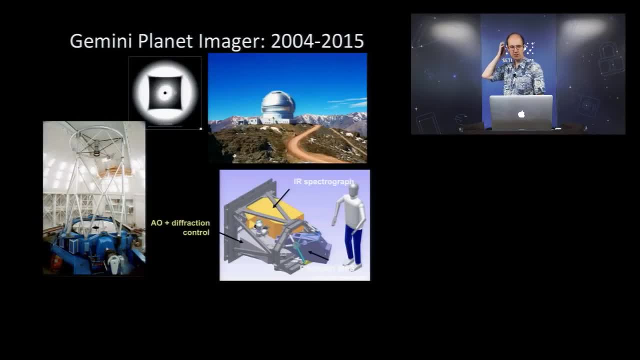 we've really got to see fainter planets down to, say, this kind of ratio of brightness, And so that's the purpose of the Gemini Planet Imager. It's an instrument whose construction we started in 2004 on the Gemini South Telescope in Chile. 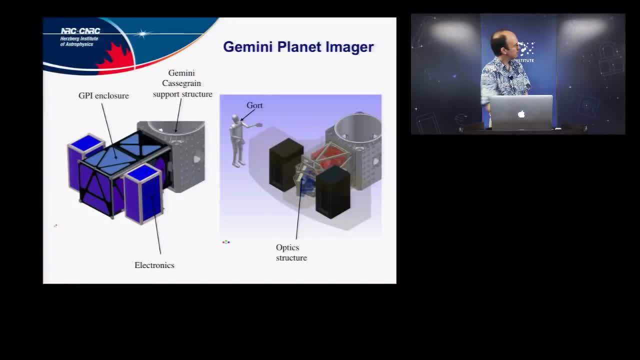 It combines a whole bunch of different pieces. I'll go through in a second. Physically, it's about the size of a person or a robot. in this case, This is the cube it mounts to on the back of the Gemini telescope. 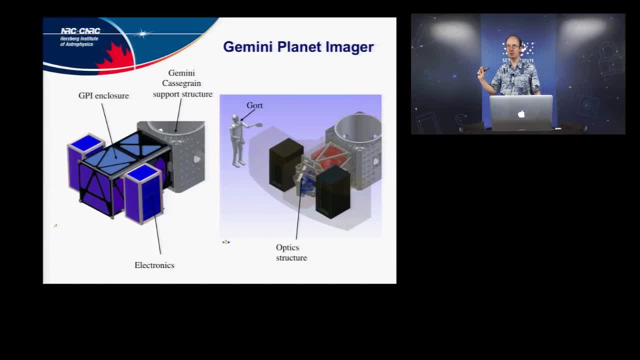 It's in a big enclosure, For example, you don't want a speck of dust on any of your mirrors because that might look like a planet, So the whole thing is in the equivalent of a class 100 clean room when it's under operational conditions. 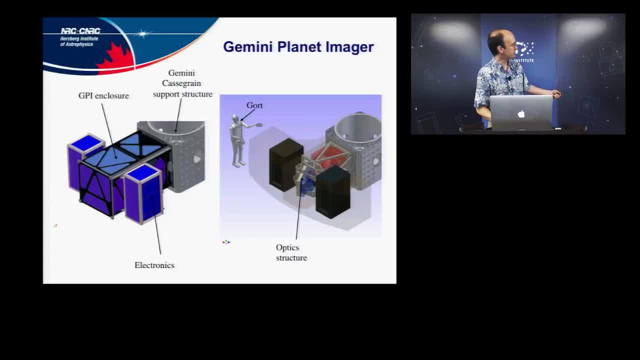 Computers that control the adaptive optic system, leave in these enclosures off to the side. Another thing you don't want is the plume of waste heat coming from a fast computer going up through your telescope and making atmospheric turbulence. So we put the computers in these boxes. 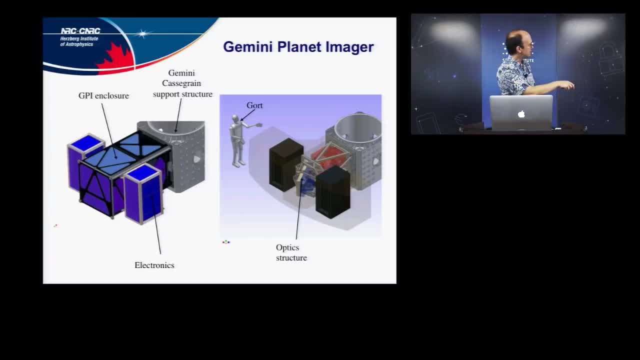 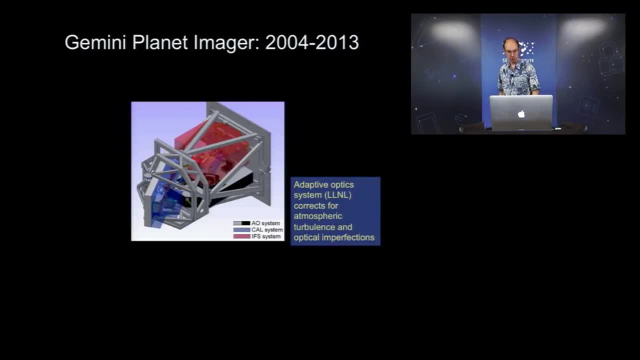 We circulate glycol liquid through the cabinets to cool them off, and then the main body of GPI lives in this interior box. It was built by a collaboration. Lawrence Livermore, where I used to work before I came to Stanford, built the adaptive optic system. 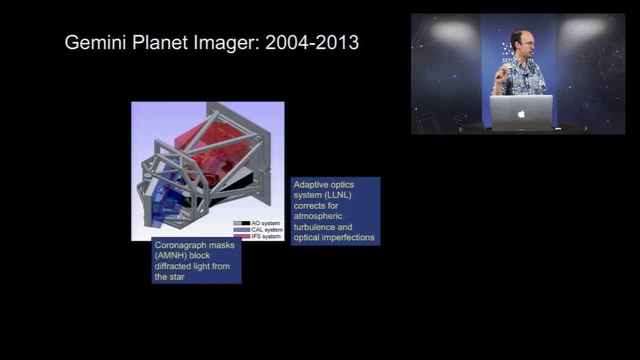 and also ran the whole project. A group at the American Museum of Natural History made some special masks to block the light from the star. I'll show those in a couple of slides. JPL built a very precise infrared sensor to measure small errors in the wavefronts of light. 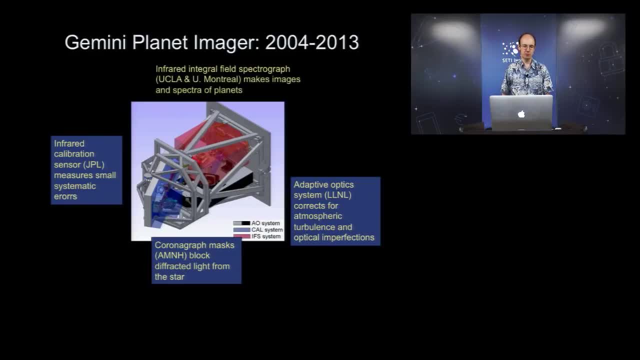 coming into the instrument. UCLA built our science instrument, which is another spectrograph like OSIRIS that makes not just images, not just spectra, but 3D spectral cubes. A group in Canada, the National Research Council of Canada in Victoria, built the mechanical structure that. 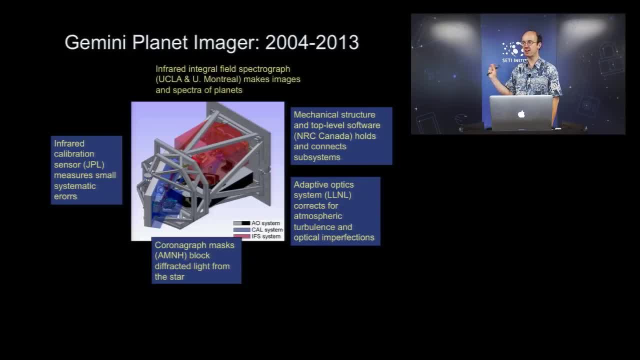 holds the whole thing together and, equally importantly, the software layers that connect all these different pieces that have to talk to each other. There's about, I would say, about 15 person years of software inside the instrument. We went to a lot of effort to super polish. 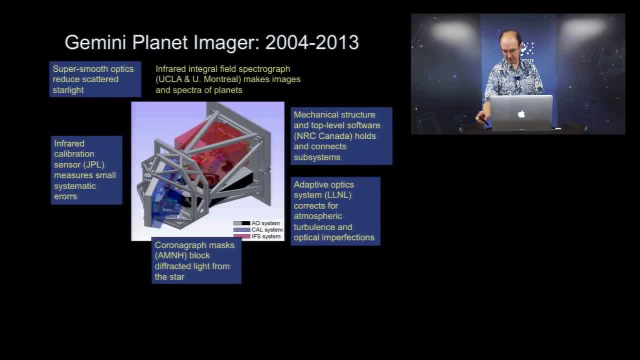 and keep all of our optics clean so they don't look like stars. One key technology for GPI to make it better than the current systems is its deformable mirror. So I showed the cartoon of a deformable mirror earlier. What a deformable mirror for atmospheric turbulence really. 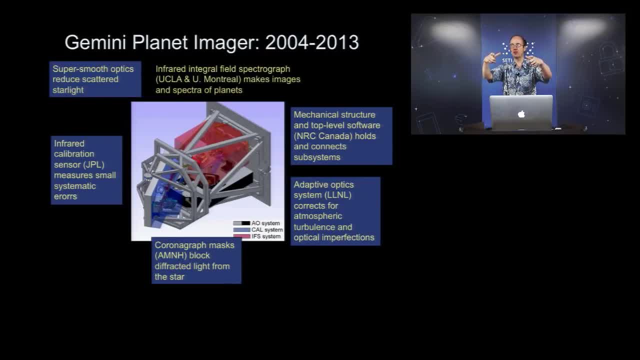 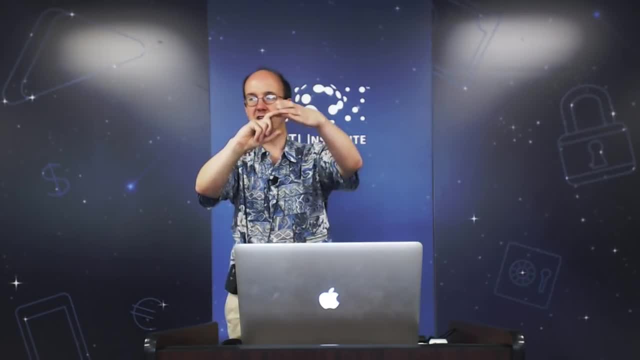 is is a thin sheet of glass- about a millimeter, so thin that you'd have to be very careful while you're holding it- maybe this big or so- with behind it a couple of hundred little actuators, little piezoelectric plungers that push and bend and warp. 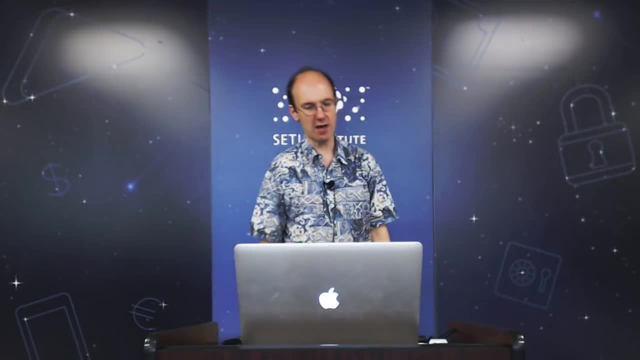 the surface of it to respond to atmospheric turbulence. For GPI we needed to do that not just at a couple of hundred locations but at several thousand to properly keep up and correct for all the little distortions in atmospheric turbulence. If we'd built this with the same technology. 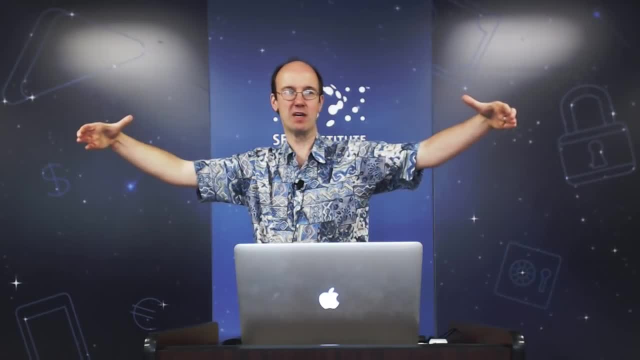 the little electric plungers glued behind it. the GPI deformable mirror would have to be kind of this big across And it wouldn't have fit in that enclosure on the back of the telescope And it would have cost on the order of, let's say, 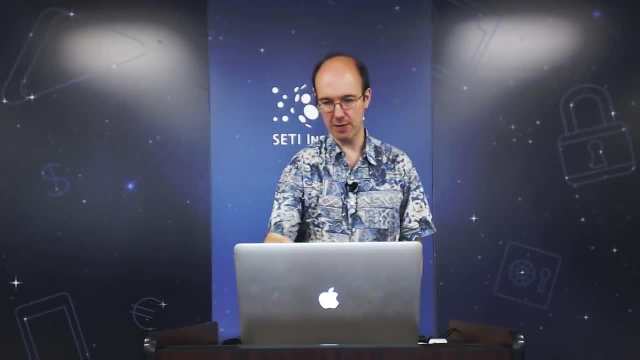 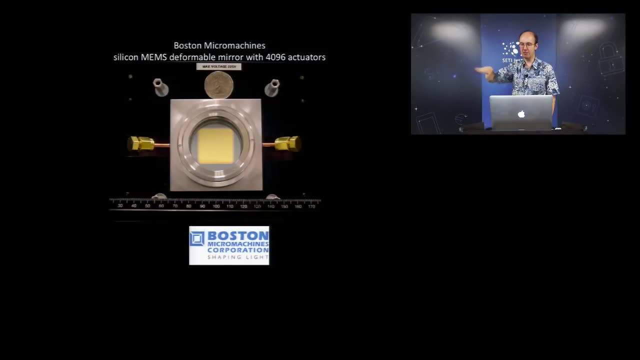 $5 million or so. Instead, our deformable mirror is actually a microchip. It's a silicon device called a MEMS, a microelectromechanical systems device, which is basically laid down lithographically the same way microchips are. 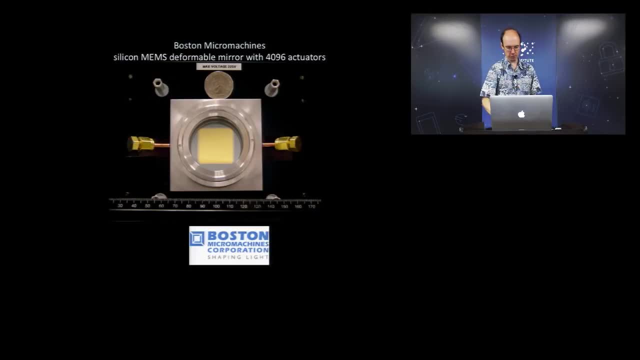 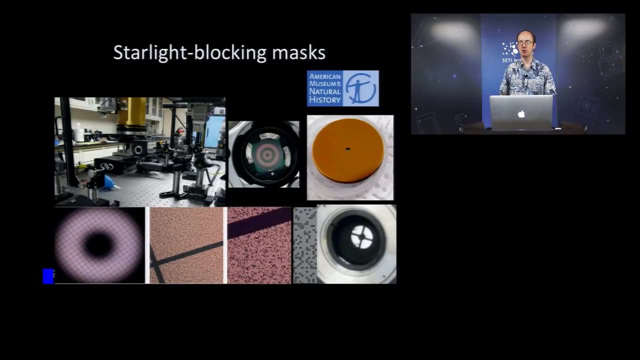 with 4,000 of these actuators in something kind of the size of a quarter. I mentioned masks to block the star. We kind of smooth the transmission of the telescope so it doesn't have sharp edges to diffract off of but kind of looks like this doughnut mask. 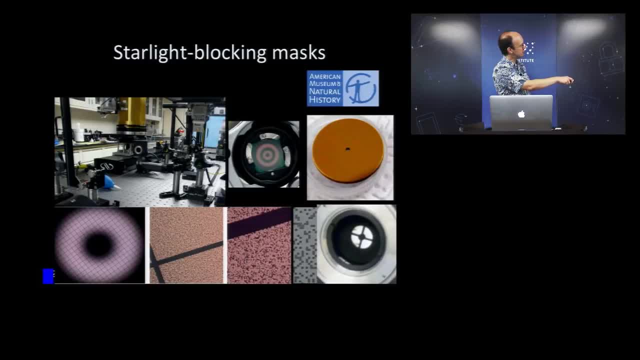 And then we focus the starlight down onto a mirror with a hole in it, such that the star falls down, The planet comes to a focus off to the side And we separate the two so we can measure the spectrum of the planet that way. 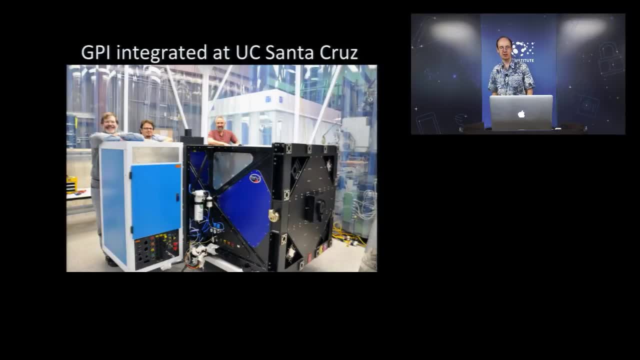 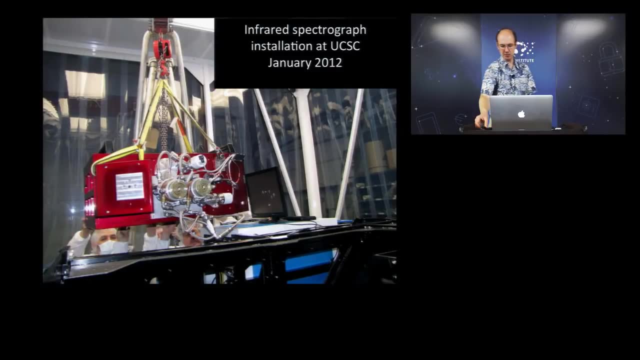 We built the whole thing at a bunch of different places, then integrated it not far from here at UC Santa Cruz. We installed the infrared spectrograph in 2012.. The instrument has to operate. It has to operate in a fairly tough environment on the telescope in Chile. 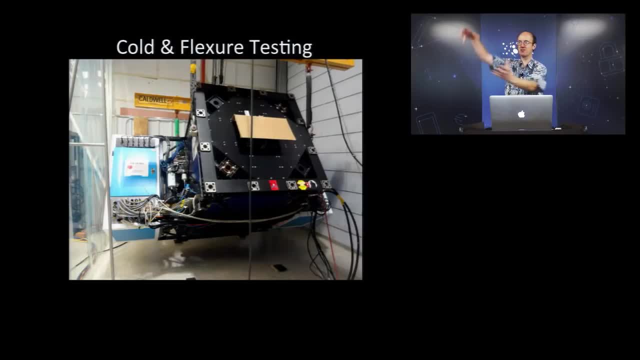 You're on the back of a telescope, So as the telescope points in different directions, the instrument might bend, And it has to stay aligned to within about 10 microns or so. So that's not acceptable. So we put it on a crane. 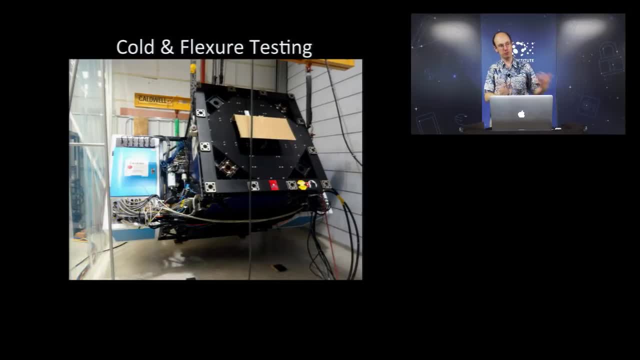 We cranked it all over the sky. We saw how aligned it stayed When it moved, which of course it does. we measured those motions And we programmed the computers to compensate for them by steering mirrors in opposite directions. Similarly, it has to work not just at room temperature. 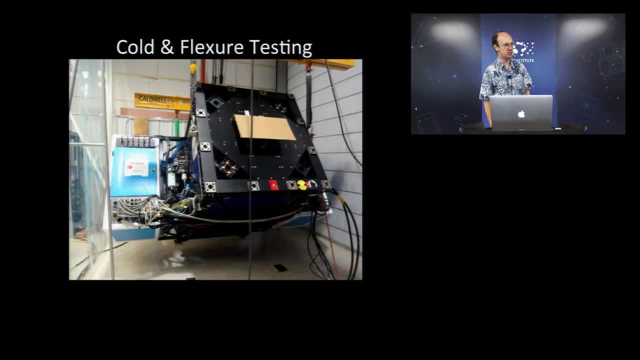 but down to minus 3 or minus 5 Celsius, which is the cold it's supposed to get at Chile. So we built a giant meat locker around it and then chilled the whole thing down to minus 5 Celsius to make sure all the computers worked. 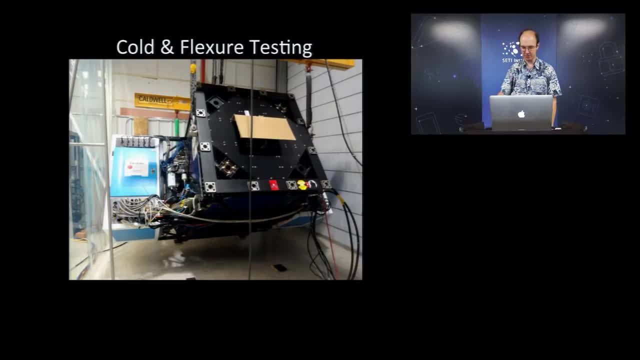 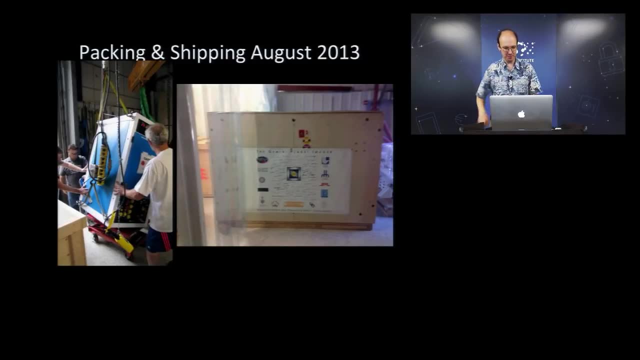 and that it would stay aligned over a broad range of temperatures. We did that successfully. We packed it up and shipped it. It's a sort of disconcerting experience to see 10 years of your life packed into crates. My small child helped with the process of packing and shipping. 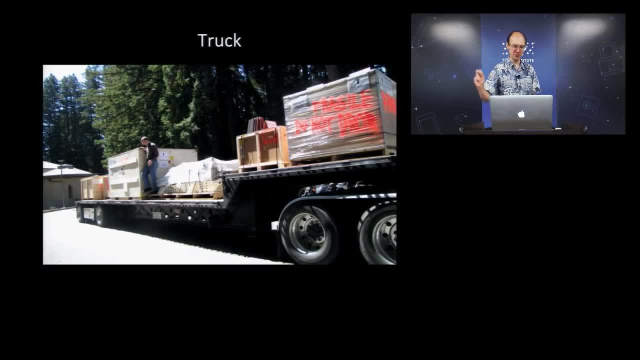 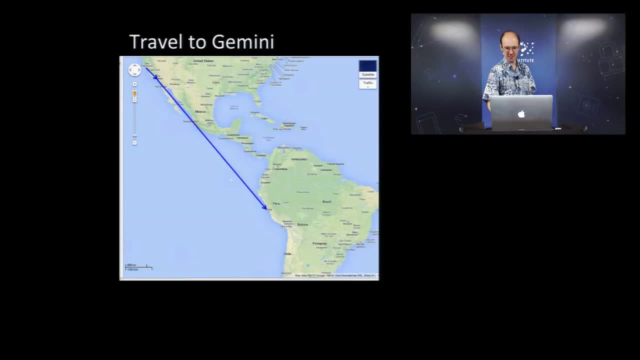 Put it on a truck You can't drive to Chile, Turns out there's no roads all the way down there. So the truck took it to Los Angeles And then a land airlines 767 took it down to, stopping briefly at Lima and then continuing to Santiago. 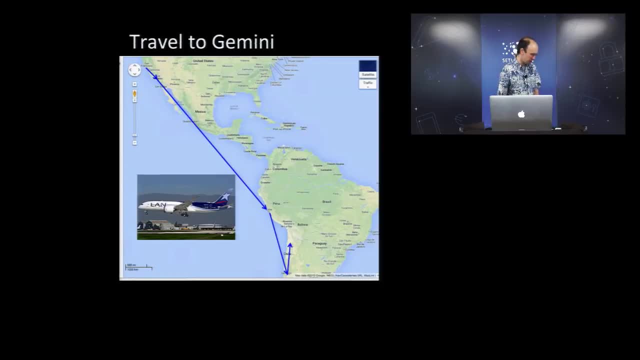 And then another truck took it from Santiago to La Serena. I did not watch this process because, first of all, I don't speak Spanish- I wouldn't have been that helpful- And secondly, again 10 years of your life on a truck. 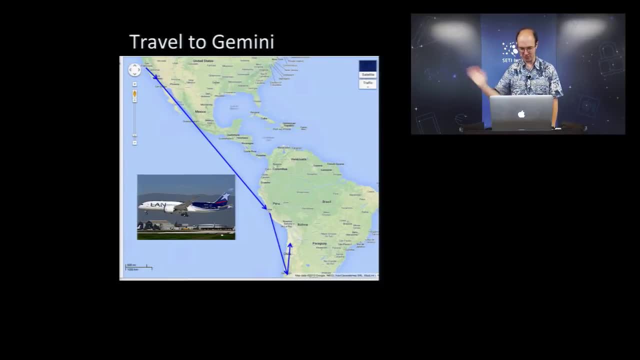 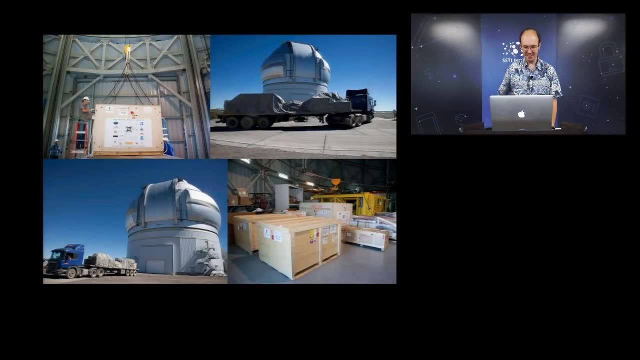 going up twisty mountain roads is. so I was just sort of heavily drugged at home until it actually was delivered. We could follow it, And it made it there intact, So it was unloaded by Gemini. There's the telescope, There's the Chilean truck. 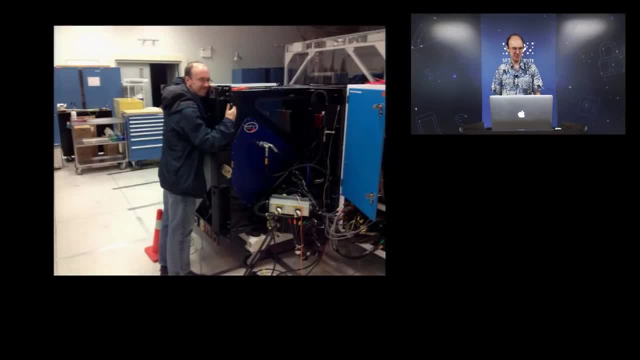 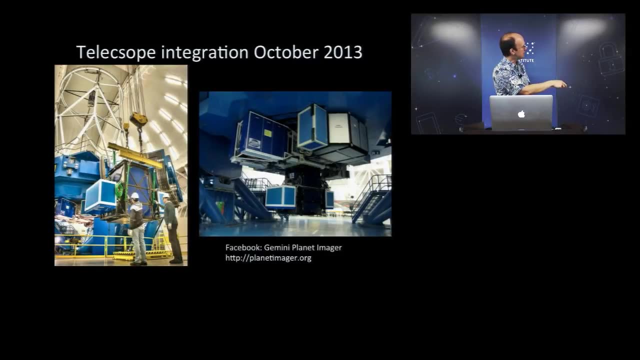 Sat in their basement for a couple of weeks. I did fly down to be reunited with it, Glad that it survived the trip. Bolted it onto the back of the telescope. A nice thing about the Gemini telescope is here. it is now on the back of the telescope, like in the diagram we saw before. 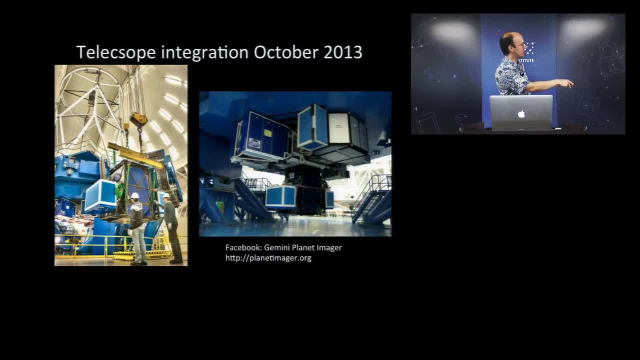 Looking up, so light from the telescope comes down into it. You can actually attach multiple cameras and spectrographs to the Gemini telescope. These are some of their other cameras and spectrographs, And so that's nice because while we were getting ours tuned up, 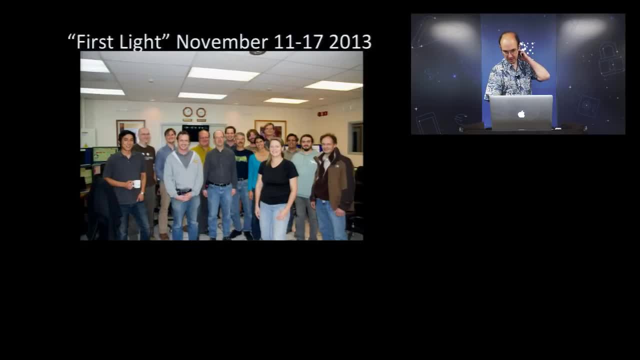 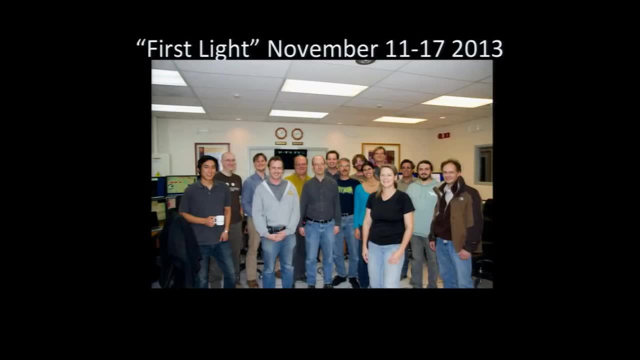 we could do science with their other instruments. Our first light almost two years ago now. Large team of scientists and engineers from a bunch of institutions down there for it. Data coming out from GPI. you'll see a bunch of examples of this, Just like with the OSIRIS instrument. it's not an image. 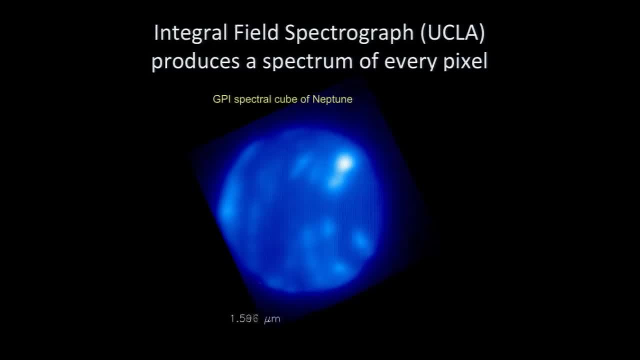 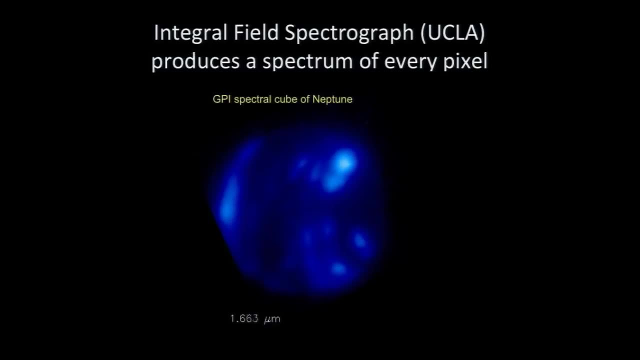 It's a spectrum of every pixel. So here's another animation from long to short wavelengths of infrared light. This is just of Neptune in our solar system. As you go through the spectrum at every pixel, we get the intensity of light as a function of wavelength. 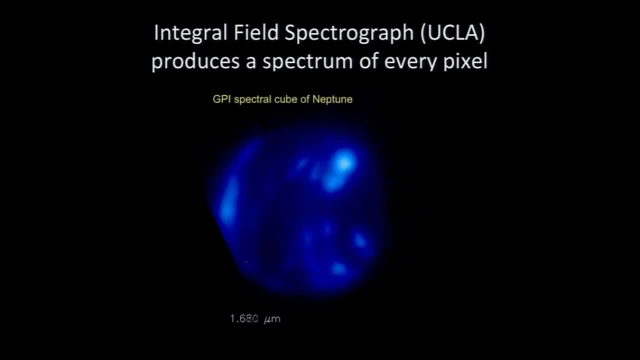 And in Neptune you can. actually We see some of this atmosphere structure. For example, these clouds here are way up near the top of Neptune's atmosphere, and so they stay bright. A cloud that's deep inside Neptune's atmosphere gets much dimmer at the wavelengths of light. 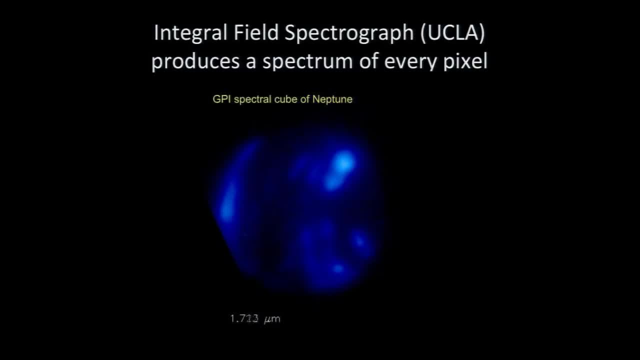 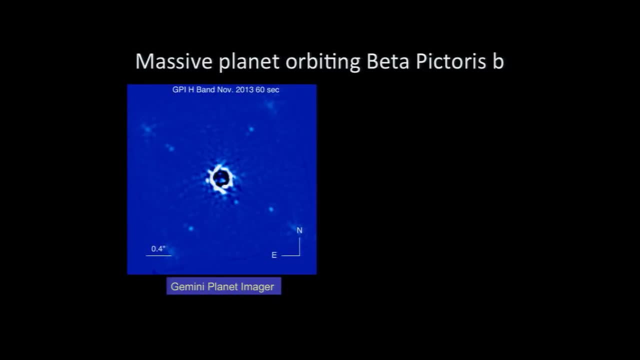 where methane absorbs, because Neptune's atmosphere is full of methane. For early GPI science, we concentrated on planets that were already known to exist. This is the planet around a star called Beta Pictoris, Beta Pic B- What you're seeing here in this GPI image. 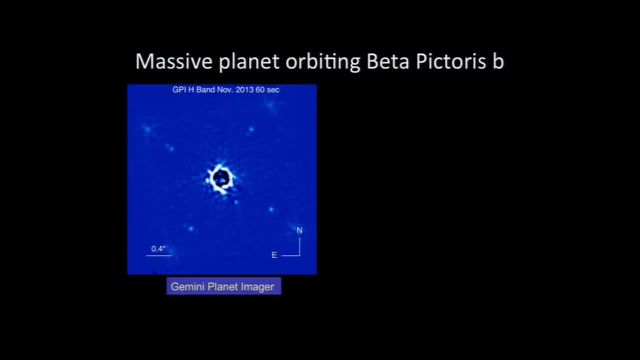 here's the mirror with a hole in it. The star fell down that hole. This is kind of a glint off the edge of the hole leftover light and diffraction coming from the star. The four spots you're seeing here are not planets. 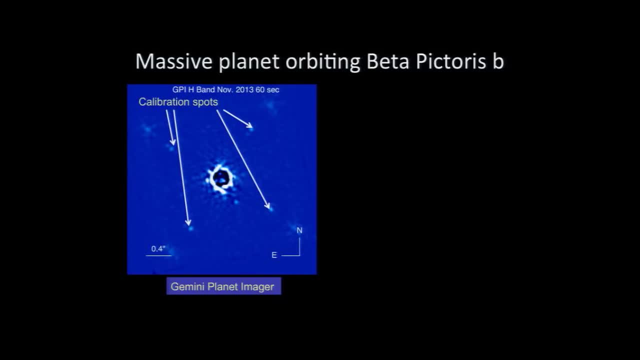 They're spots that we induce in the image as a calibration, And the reason we induce them is that, when you find a planet, one thing you'll want to know is: how far is it from the star If the star disappeared because it fell down the hole? 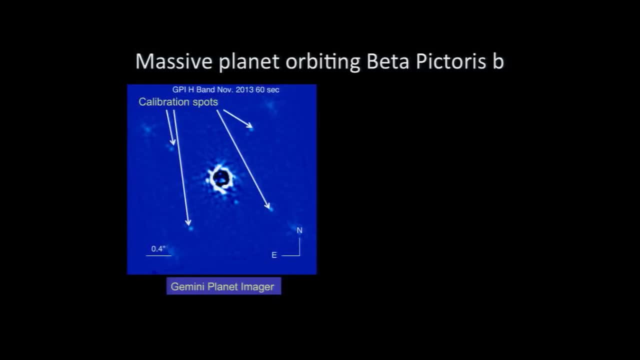 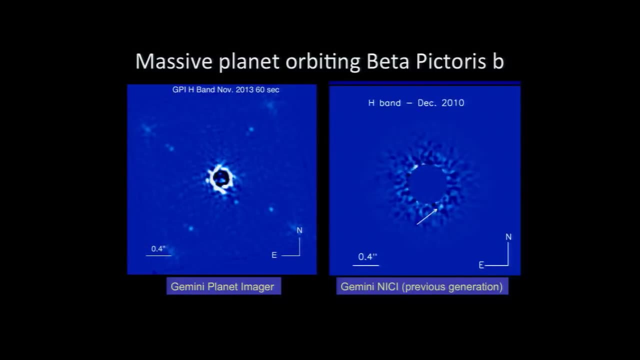 that's hard to measure. These four spots are actually lined up so that the intersection of them is always where the star is, so you can trace the star position very accurately. The planet is that little dot here, So that's another big one, about 10 times the mass of Jupiter. 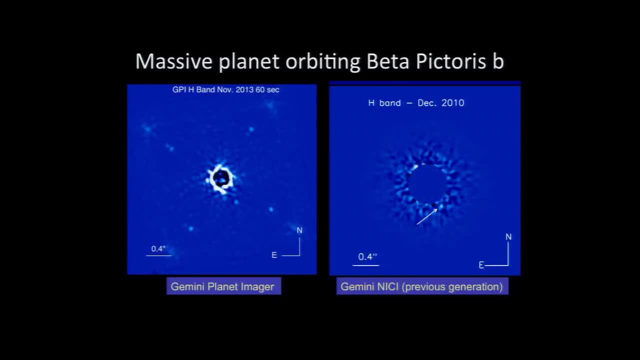 For comparison, here's an image from a previous generation instrument: the people who discovered that, not the people who discovered that planet- another group After it was discovered- planet's visible. planet's more visible in the GPI image, so we're somewhat happy. 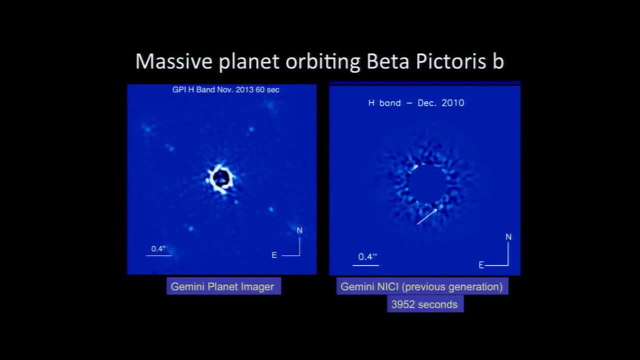 But we're extremely happy because this took 3,952 seconds of telescope time, and that took us 60 seconds of telescope time to make the same image, So GPI is, in fact, substantially more sensitive than its predecessors, And so we were happy. 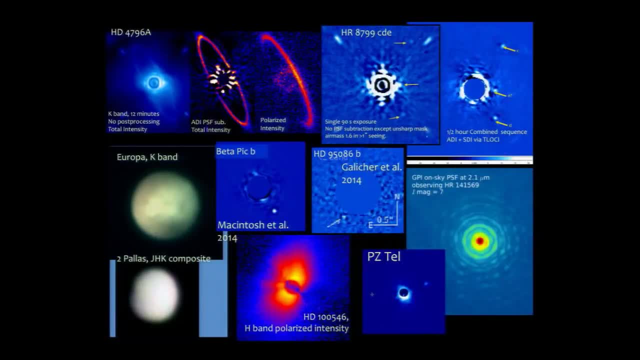 So GPI has looked at a wide variety of objects. I think James talked about some of them in his talk- I don't have time to discuss it in detail- including disks of asteroid or comet material, orbiting stars, Europa and Pallas. some images that Frank looked at: 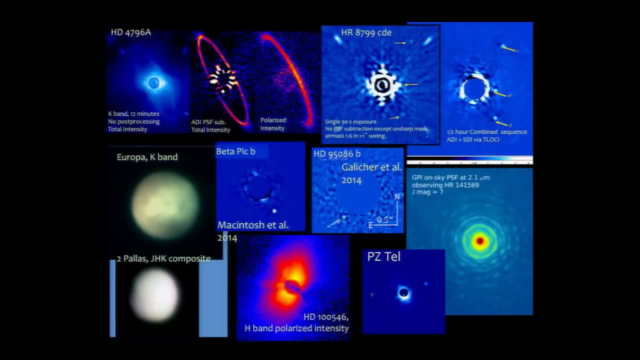 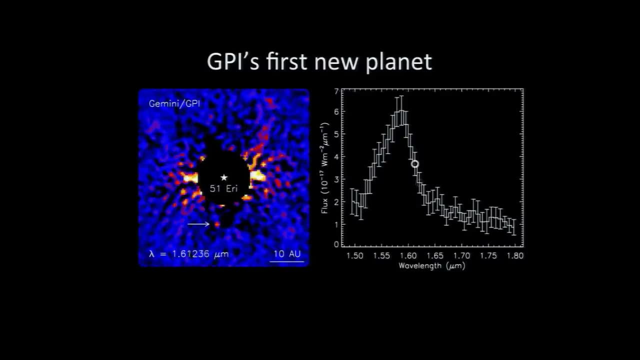 young disks that might be in the process of forming planets. a whole bunch of other planets people have known, But what I'm here to finish up about is talking about our first new planet. So here's another one of those spectral cubes. I should get a version without the arrow. 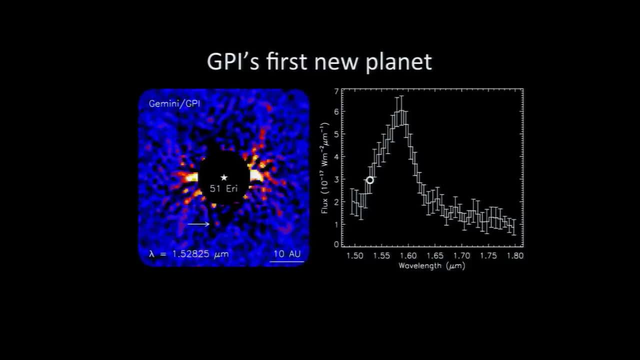 to see if people can spot the planet. because what happened literally was we started looking for new planets in November of last year, So we're targeting a population of young stars- about 600 of them- to see which have nearby planets. We had an observing trip in December, right before Christmas. 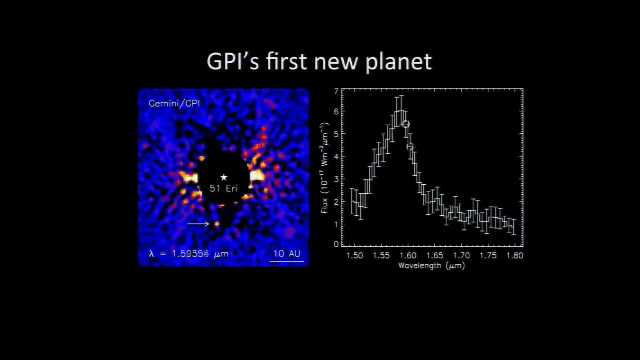 All of us went home pretty much except for one grad student and one postdoc at Berkeley. And the postdoc, literally looking over the grad student's shoulder at a computer in Berkeley, saw a little dot that was kind of coming and going. 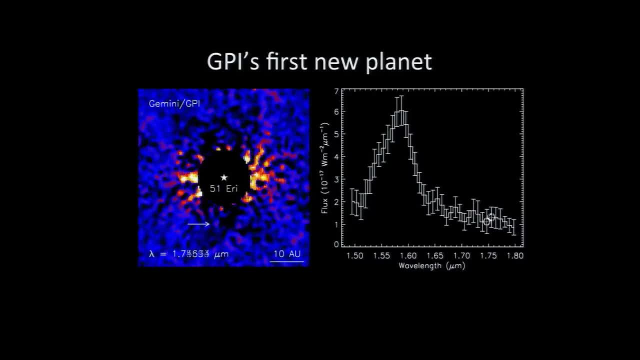 All these artifacts sort of hold still, but this little dot is coming and going because the brightness of the planet is changing as a function of wavelength, And here's its spectrum And it's changing exactly the way our model said cold planets should, where light is being absorbed by methane. 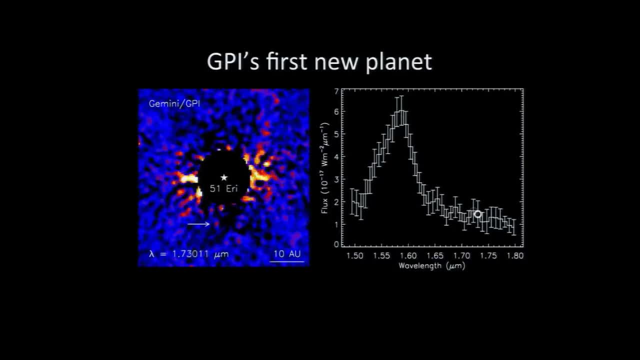 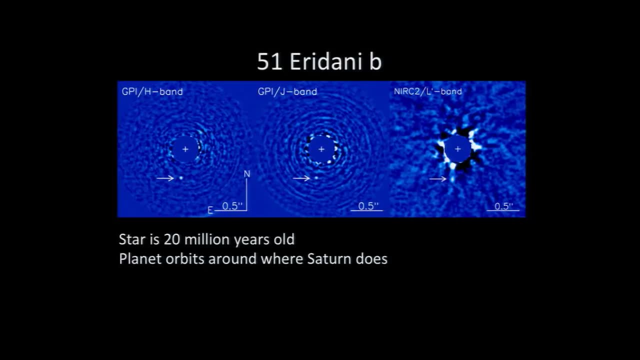 and emitted by the hot clouds deep in the interior of the planet. The star is about 20 million years old. If it's really a planet, it would be orbiting around where Saturn does, And so the first question we asked ourselves is: 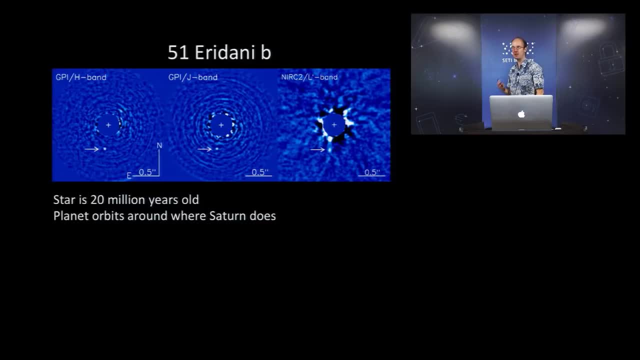 is it really a planet? It turns out there's a large history of thinking you found a planet and being wrong in this game for a lot of reasons. One of the most popular reasons is what we see here. here's the images from GPIE again, and a Keck image. 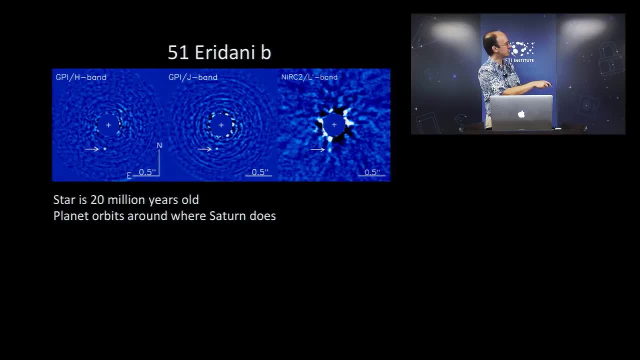 We actually took an image with the Keck telescope, so at least we know it's not an artifact from the telescope, because it's there with Keck as well. You see something very faint next to something very bright like a star. One explanation is you're seeing something very faint. 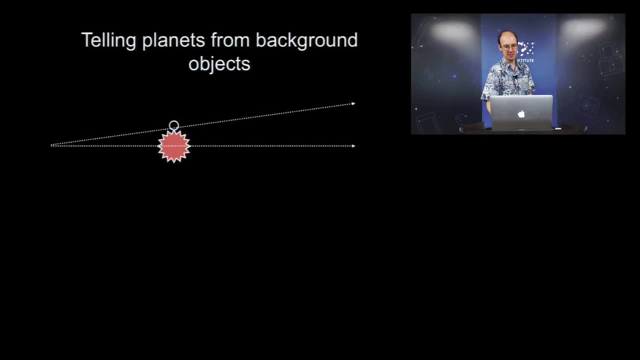 because it really is very faint. It's a planet right next to the star, and planets are faint. Another explanation is it's very faint not because it's really faint, but because it's very far away. It's another star that, through an astonishing coincidence, 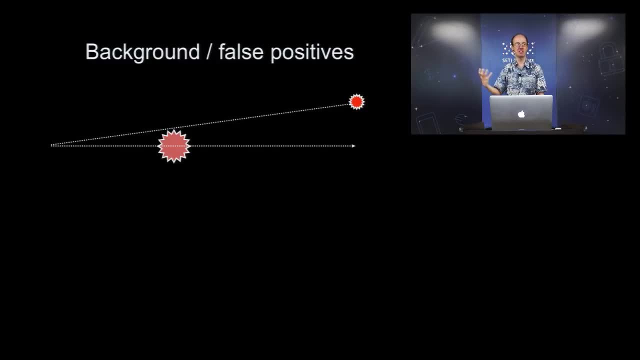 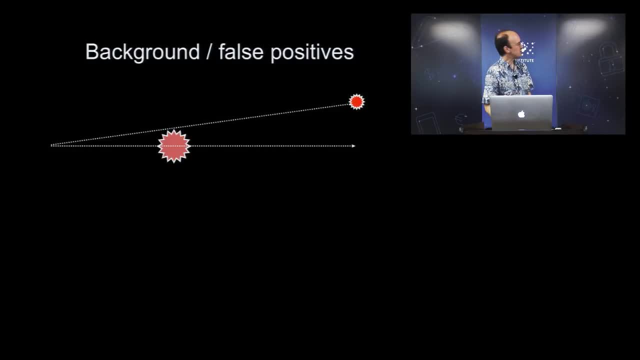 over the course of the career. So traditionally what you do is you come back a year later and you look for motion. If it's really a planet, it'll move with the star, plus maybe orbiting around the star If it's really a background object. 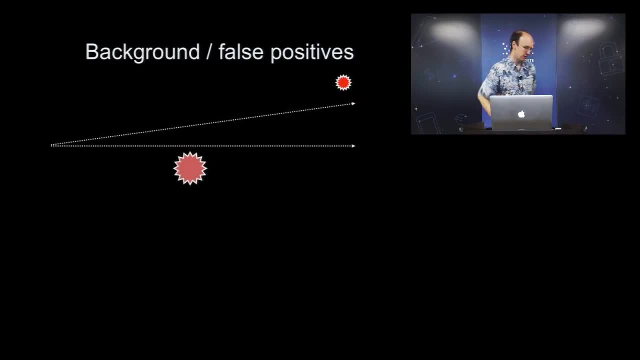 it'll either hold still or wander off in some separate direction. We didn't want to do that, partially because we've been doing this for a long time and we're not very patient, but also partially because we didn't think we needed to. 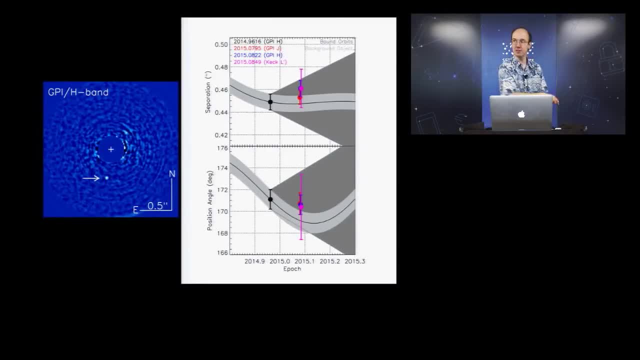 We did observe its position at multiple eras. This is a graph Eric Nielsen here at SETI put together. Here's the year versus the position of the planet. When I plot these, I plot the separation between the planet and the star. That's the top one. 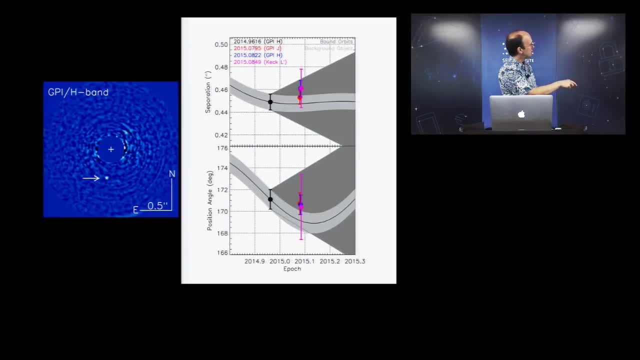 And also the angle that the planet and the star make. That's the bottom one. We saw the planet in December of 2015.. We confirmed it after Christmas, in January of 2000 and, excuse me, December 2014.. January 2015.. 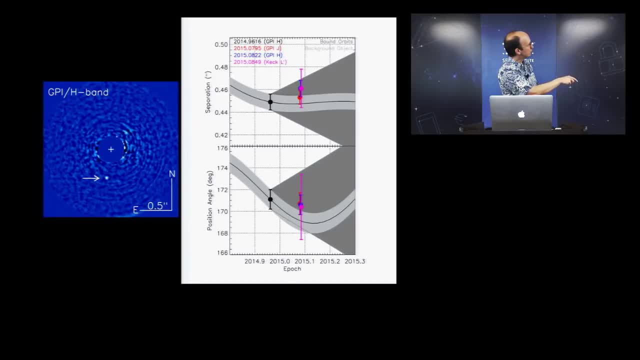 But that's such a short period of time. The gray track is the path a background object would have followed. The cone is the range of orbits a real planet could have followed And you can see, over this short period of time there's no way to tell the two of those apart. 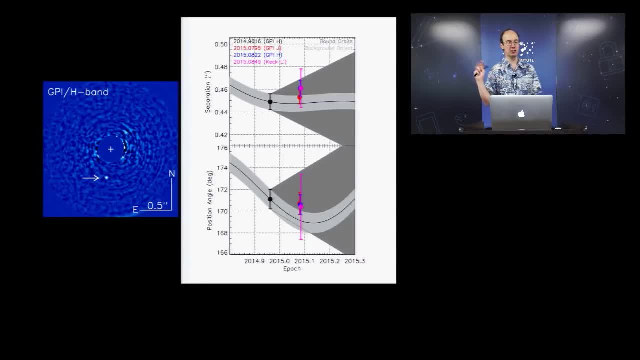 We did dig through a lot of archives and we discovered half a dozen other groups had looked at this one individual star to try and find planets. None of them had seen it. of course They would have published it. We took, for example, some old Keck data from 2003.. 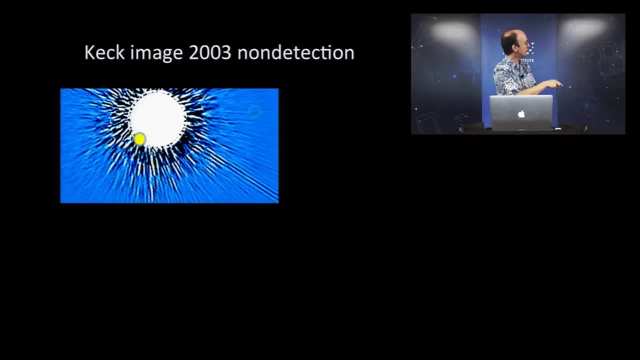 We analyzed it very heavily to see if we could see the planet which would have been about here. We couldn't see the planet. It makes sense Keck is less sensitive than us, But that does actually help us tell if it was a background object. 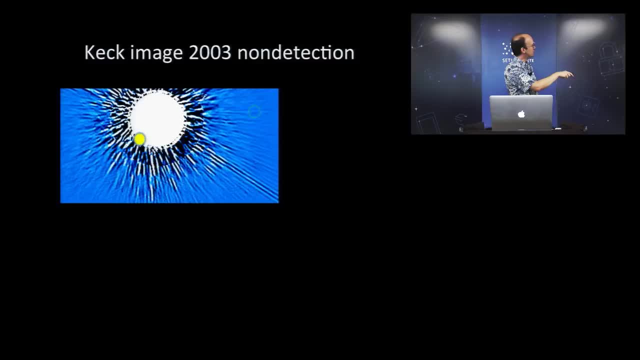 The star is moving kind of this way, And so if it had been a background object, the star would have left it behind, It would have been farther away from. excuse me, the star is moving towards the planet. So if it had been a background object back in 2003,. 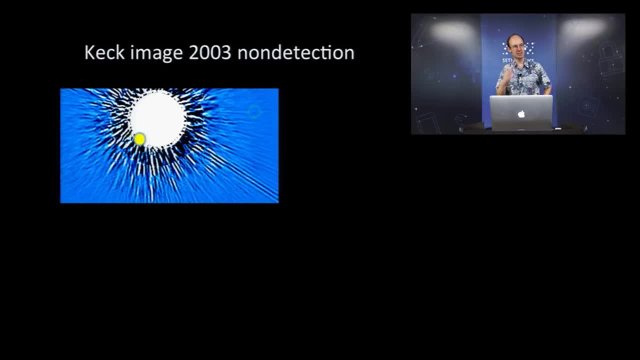 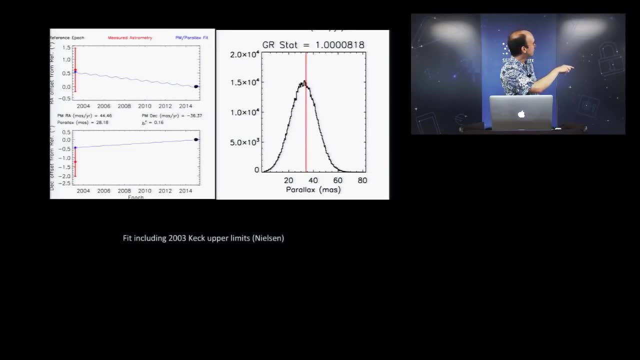 the star would have been further away and would have been just barely detectable by Keck, And in fact we can sort of exclude a range of allowed motions for it. This is a plot, again Eric put together, of now the separation between the planet and the star. 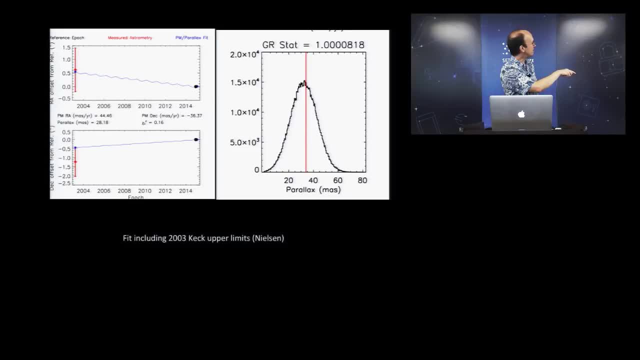 We know, way back in 2003,, the planet had to be within this range, not right on top of the star. We know where it is now, And so we can partially constrain the fact that it's not at least a stationary background object. 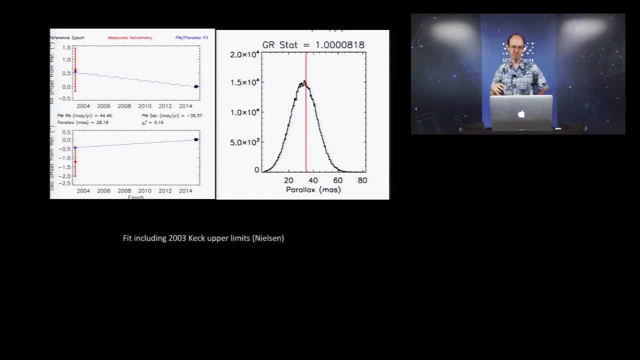 So that helps, But it could be a background object that's still moving And in fact the referee on our paper said you should re-observe this for you. It was this very snarky about: this is the gold standard. 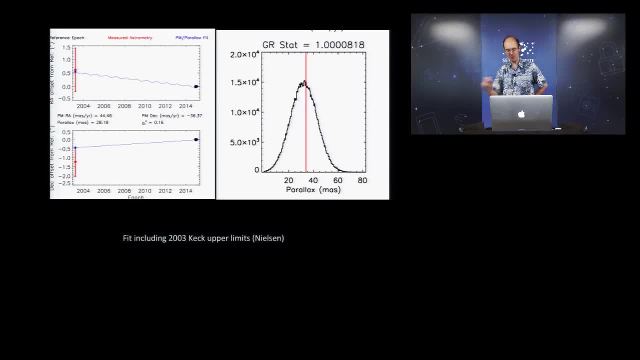 And if people publish a paper that doesn't go up to the gold standard in science, they may be right, they may be wrong, But it'll be a bad example for the kids And everybody else will be publishing planets that aren't really planets. 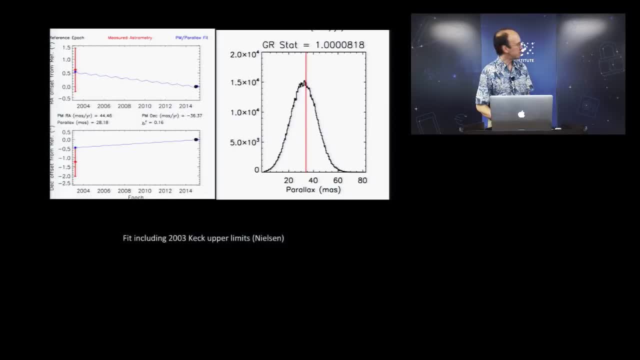 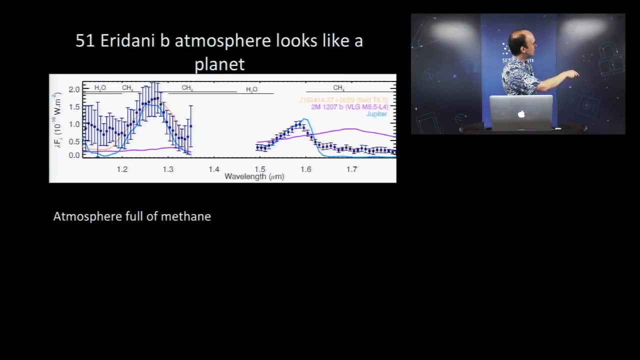 We did not find that compelling as an argument. What we did find compelling is that because it's GPI, we have a spectrum And stars don't look like planets. Here's the spectrum at short and longer infrared wavelengths And it's got this enormous signature. 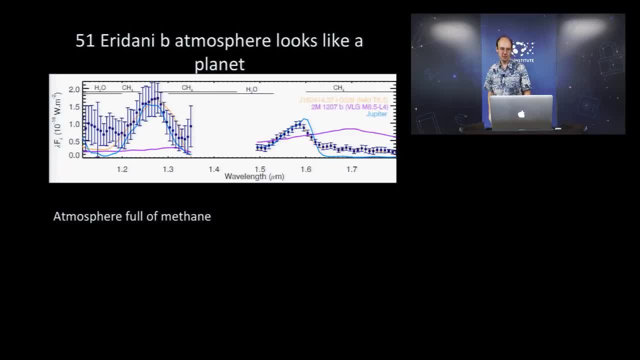 of absorption due to methane. Stars don't have methane in their atmosphere. What does have methane in its atmosphere are either real planets or things called brown dwarfs, objects that are in between planets and stars, And the thing about the brown dwarfs is they're incredibly rare. 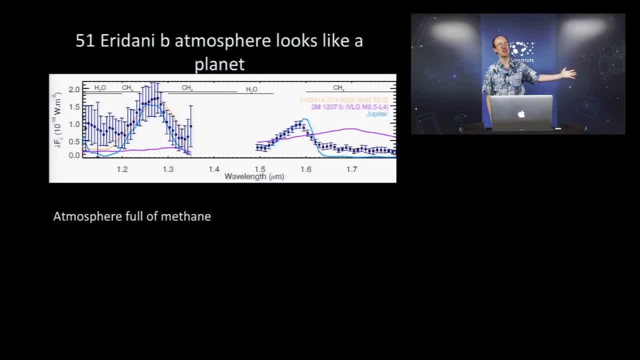 The odds that you would get a brown: to find a brown dwarf you have to survey pretty much the whole sky and you find 100 of them. The odds that you'd find one right next to your individual star: nearly zero. And in fact, the most compelling, not the most. 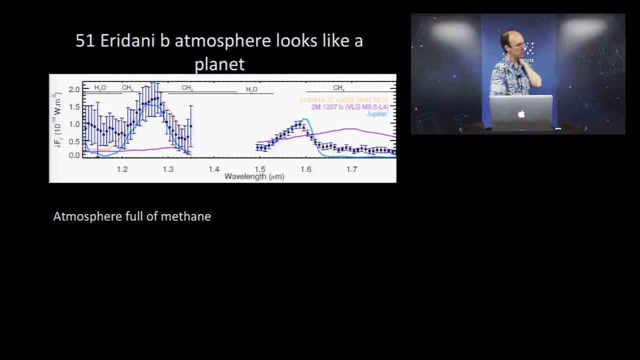 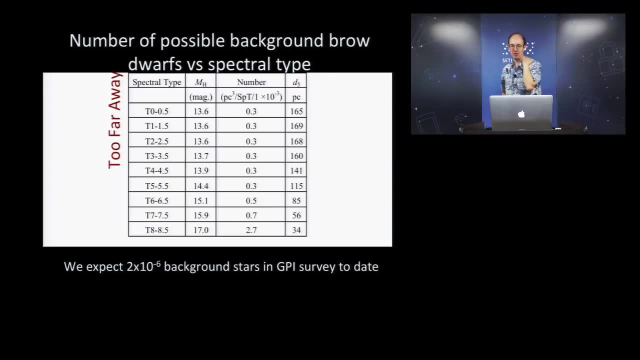 compelling quantitative argument. we did the calculations and we say that there'd be about one or two per million stars. we look at background objects that we would actually find, So the odds of it being a background object are relatively small. An example of that is that a whole bunch of other people 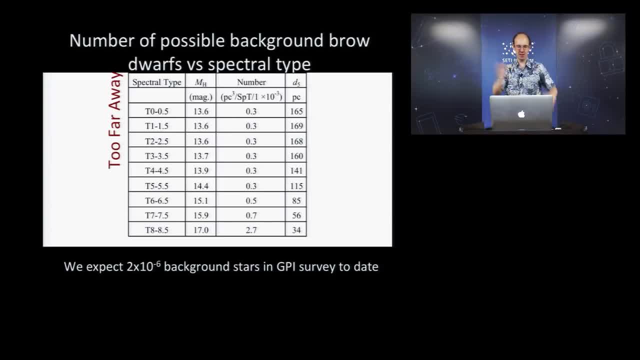 looked at this star to see if it had a planet or not. They looked at it with cameras with huge fields of view that have just as likely as we are to find background objects, In fact, more likely, The only place we can look that they can't. 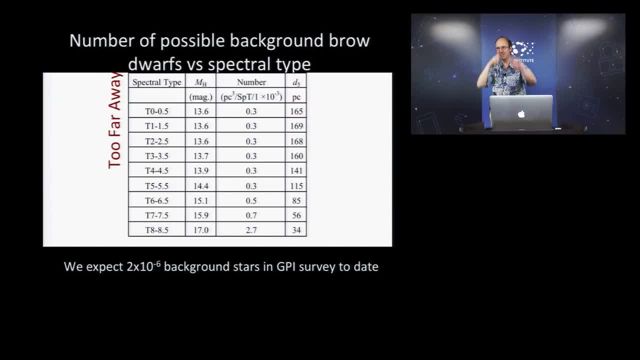 is right next to the star. Background objects should be anywhere- planets right on top of the star. So the fact that we found it with a planet image, or it even says that on the label, means it must be a planet It's. I won't go through as I'm running low on time in detail. 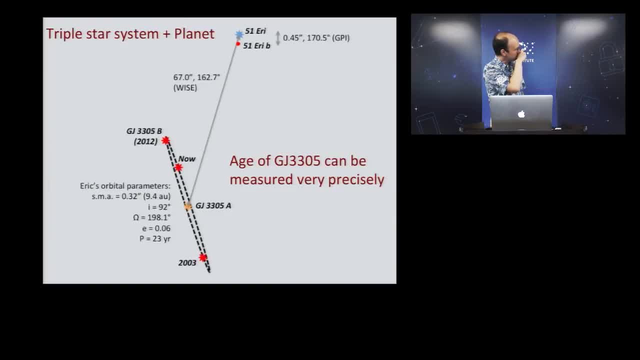 but we know the age of the star very precisely because it's actually part of a triple system. Here's another figure Eric put together: The star and its little planet are over here, and then there's another pair of stars that are orbiting around them. in this complicated ballet. 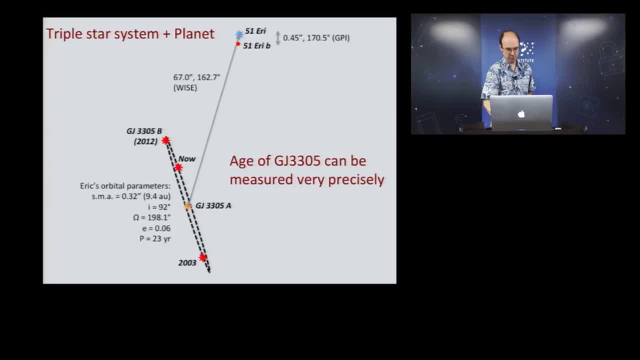 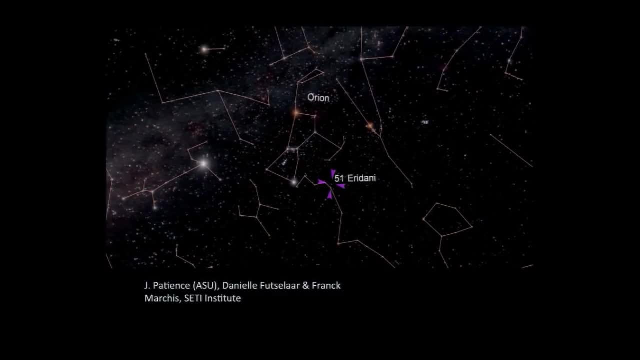 This pair of stars. they're relatively low mass stars and you can measure their age very precisely. We did put together a very cool animation: Jennifer Patience, faculty at Arizona State University, together with her planetarium, and Danielle and Frank working through here. 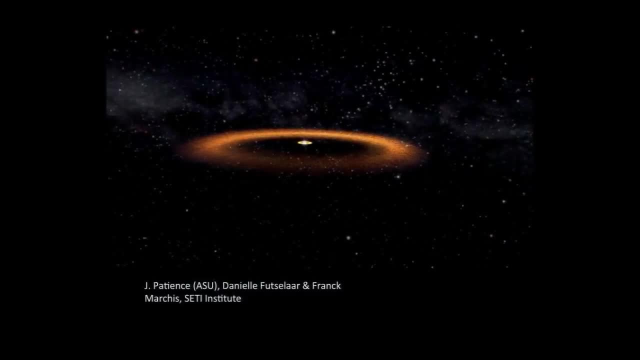 They put together an animation showing the system. Like HRD799,, this system has a comet equivalent belt and an asteroid equivalent belt and the planet is kind of in between them, which is probably where planets should be. As we zoom in close, you can see the planet. 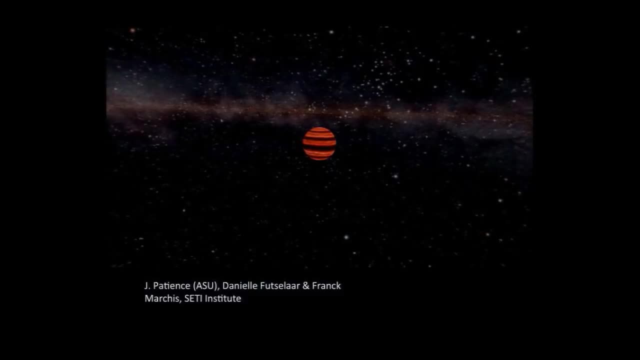 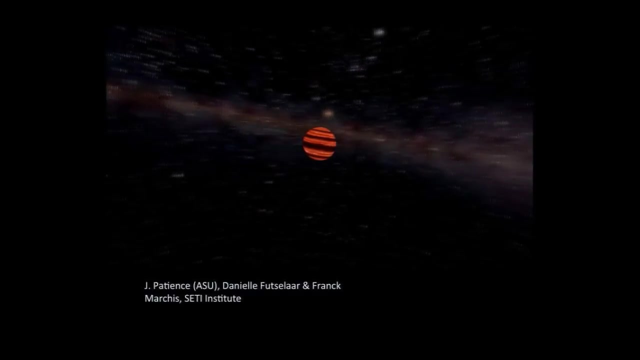 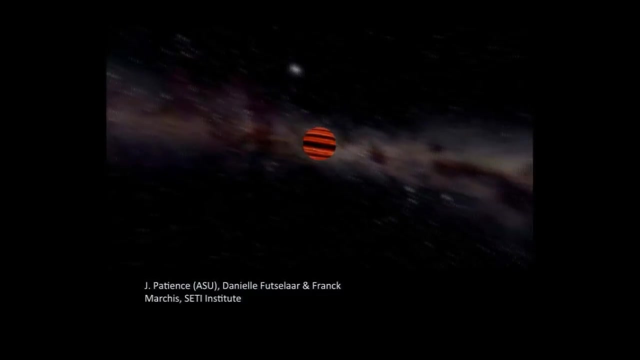 sort of sitting there, Jupiter-like, but glowing, because what we see is the infrared glow from it, And in this figure as it zooms around, you can also see the other two stars in the system. I don't actually know. Frank might know if they got the orientation of the Milky Way. 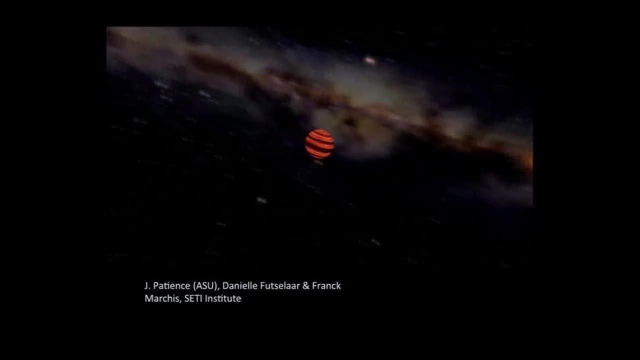 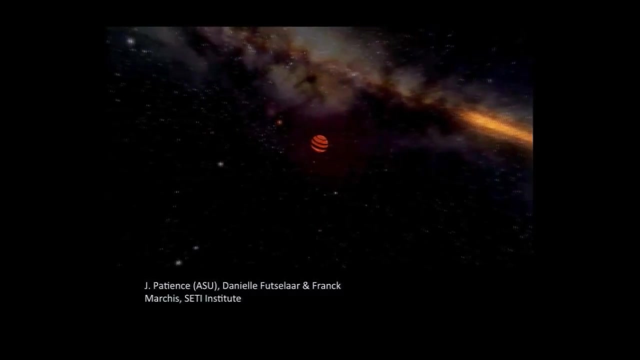 right or if this is just arbitrary, But it doesn't really matter. Missed the double system. All right, I should have pointed it out. I said you should be distrustful of all these gratuitous artist conceptions, which is sort of true. 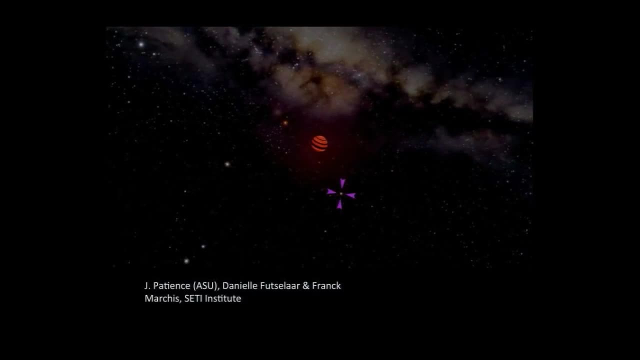 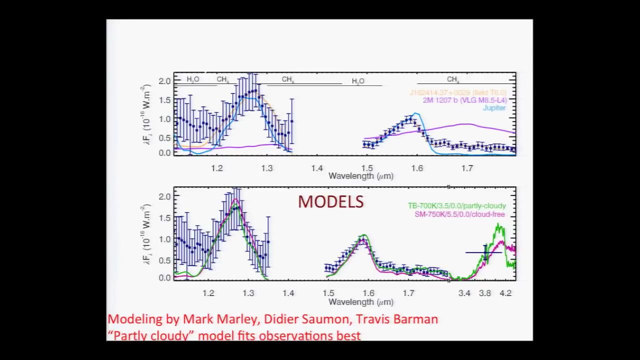 But we don't have an image that looks like that. We do have this spectrum, And from this spectrum you can take models that tell you things like what the surface is like, what's it's like, What the atmosphere is like. excuse me, 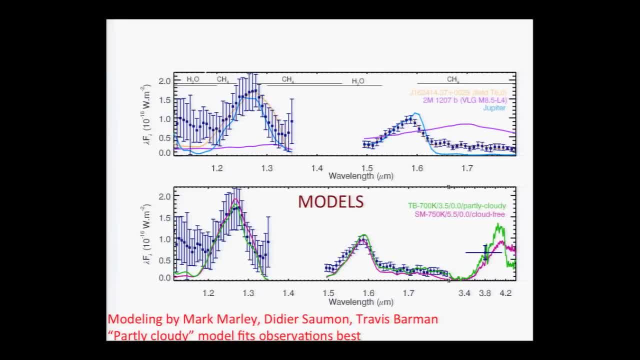 And in order to reproduce the bumps and wiggles in this spectrum successfully, we have to have an atmosphere that is kind of half covered by clouds that are cold at the top of the atmosphere, but half without clouds where you see deep into the hot interior of the planet. 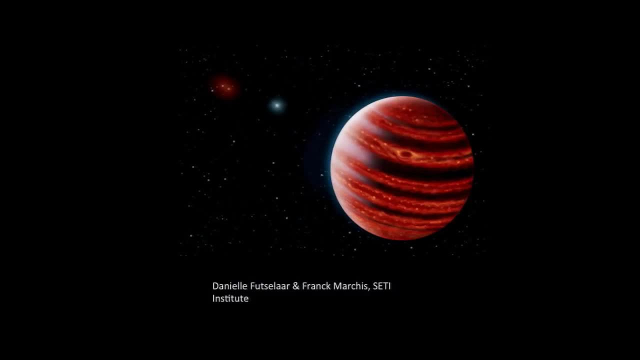 And this artist's conception that Danielle and Frank put together actually reflects that. So I don't know in detail that there's five bands or seven bands. I don't know that the bands are elongated or there's a giant red spot, But I do know that, if you were to look at this planet, 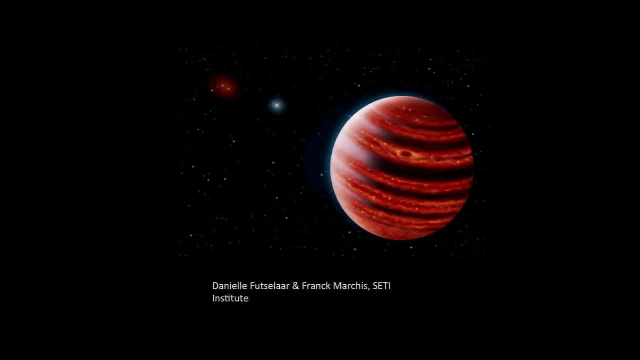 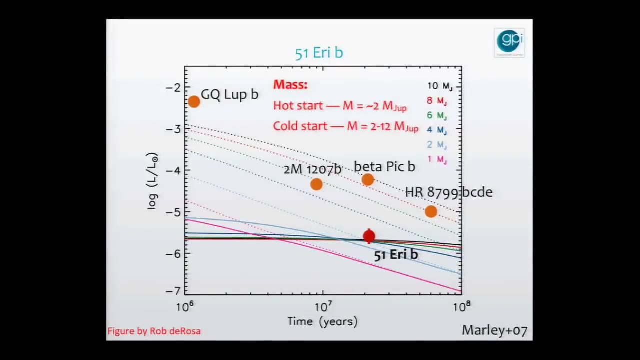 with your eyes, you would see a surface that's sort of half glowing deep in the inside and half dark and opaque clouds on the top of the atmosphere. And then finally, in terms of its formation, this is sort of the first planet that could have formed. either way. 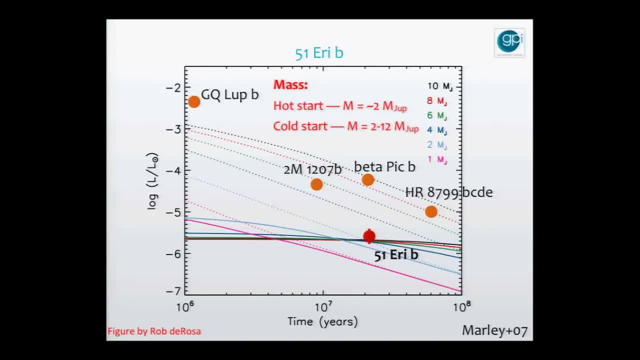 Here's another version of those formation graphs: brightness of planet versus time. All the previously discovered planets are way up bright where hot start planets could have formed. This one is sitting a little bit under a million times fainter than the sun where potentially a planet that formed. 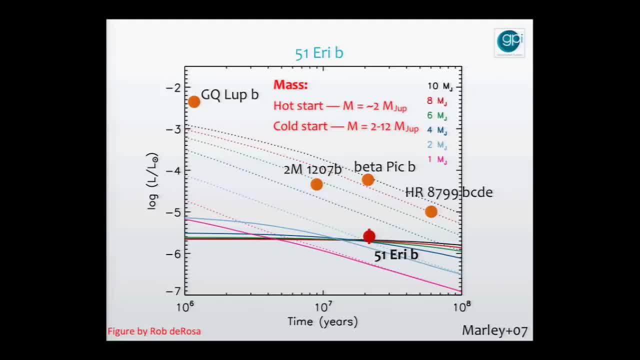 like Jupiter would be sitting at this age on this particular graph. We can't tell for sure. It could be a very small planet that formed hot and just isn't bright because it didn't have a lot of energy to start with. It could be a big planet that formed cold and is not very 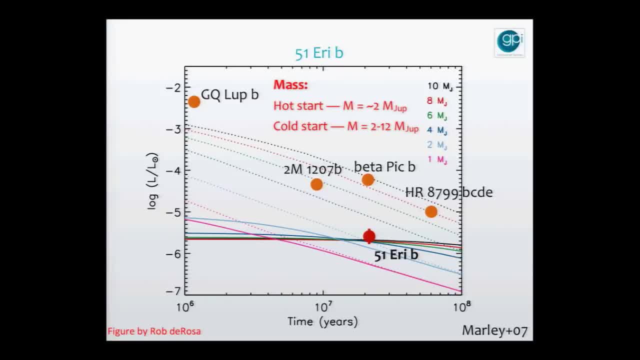 bright because it lost a lot of its energy forming as its core, as it accreted mass on its core. But someday we may be able to tell the difference If we could ever measure the mass of the planet, and there's some hope that in five years. 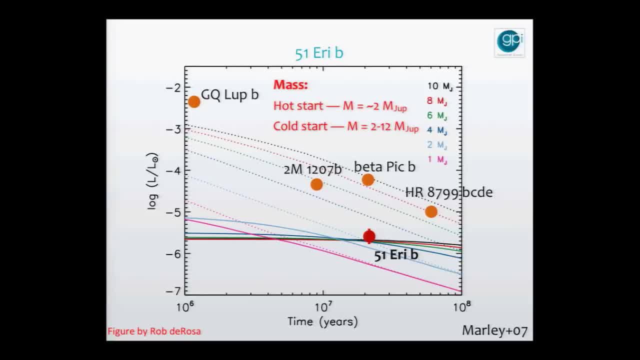 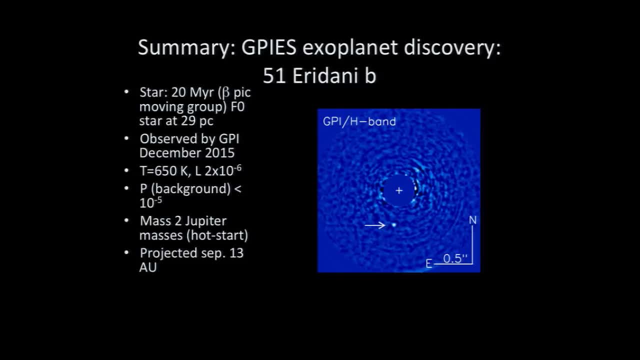 we might be able to do that accurately. we could tell whether it sits on this hot start or cold start family of curves. So, to summarize, it's about 20 million years old. We've seen it since. it should say December 2014,. excuse me, 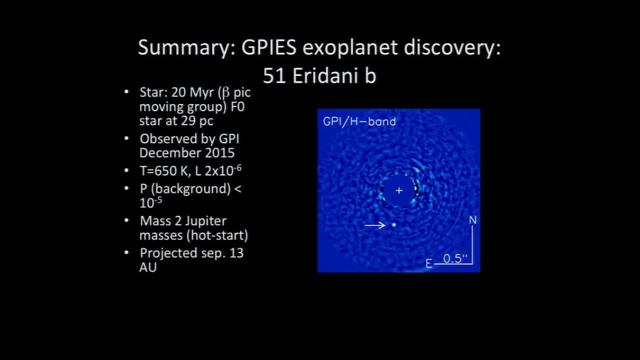 Temperature about 650 Kelvin, 2 times 10 to the minus 6, the brightness of the sun. The odds of it being a background object are less than 10 to the minus 5.. The mass might be twice the mass of Jupiter. 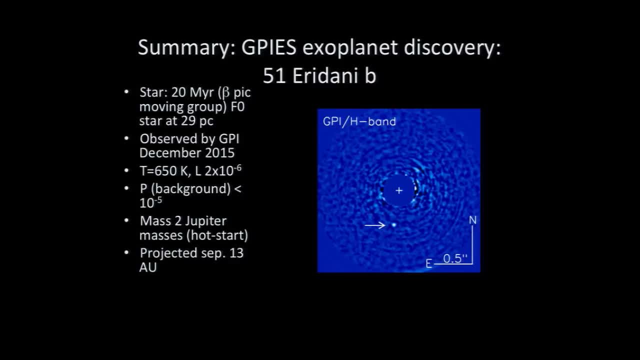 at a separation of Saturn, Not quite our solar system, but getting there and young enough that it remembers how it formed. And then, just as a hot off the presses, I was in Chile. What day is it? I was in Chile a week ago and we saw that the planet is still. 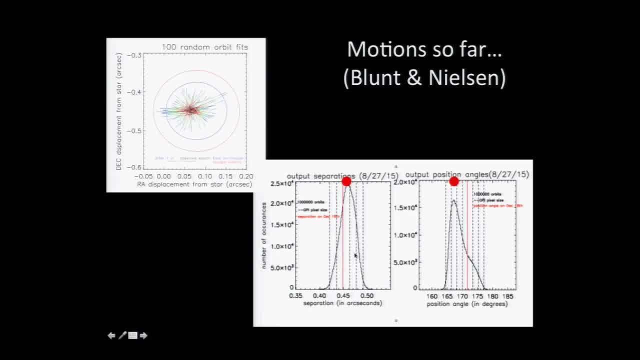 there, Which is kind of reassuring. Before we went there, Eric and his summer student, Sarah, did some modeling of the range of motions it should have. It's actually pretty close to where the range of motion, where the predictions say its motion should be. 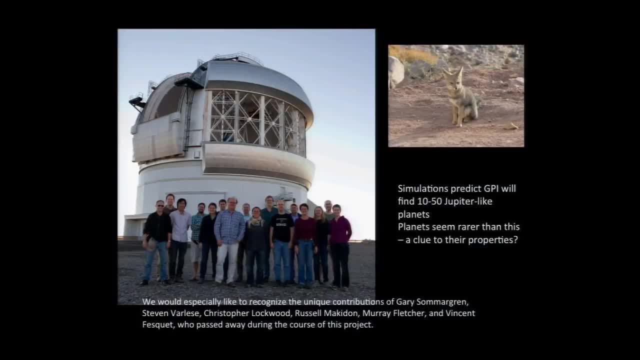 And over the next six months we'll be studying it in a lot more detail, And so I think I'll finish there rather than going into the space mission stuff. But I'm happy to talk about future space missions to other people. Hi, Bruce. 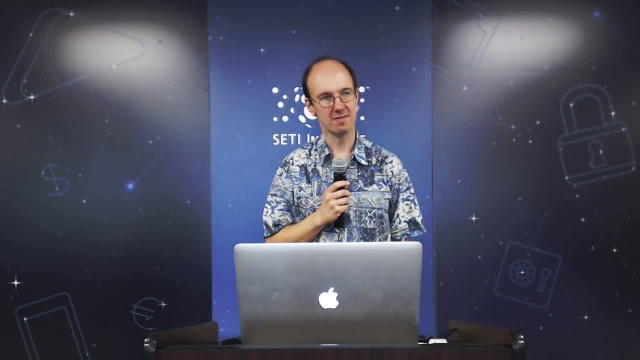 Nice talk. So my question is: what are the chances that GPI would be able to image a planet by reflected light rather than self-luminous light, Say Alpha Centauri or something like that, Not to put too fine a point on it? 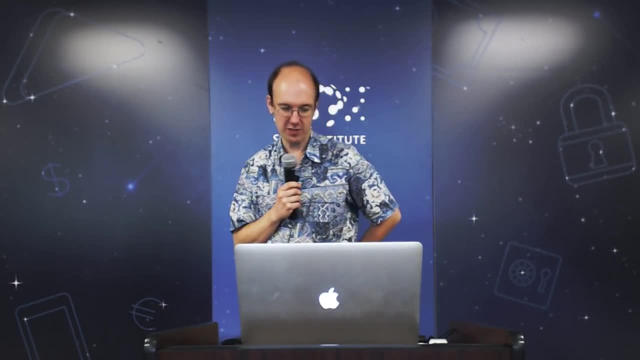 It's right, Russ kind of knows the answer to this, but it's a good question to ask, And GPI wasn't designed to do this. It was designed to look for the self-luminous planets. The signal from a reflected light planet is very small. 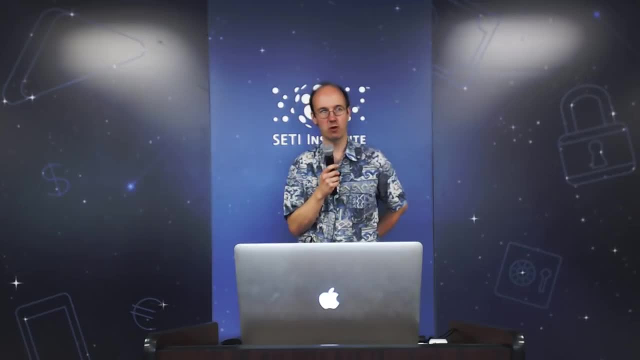 but not completely out of the question, And especially if you took advantage. you took advantage of polarization. So one capability GPI has that I didn't talk about at all is it can measure the polarization of light as well as its spectrum- Light that's scattered by turbulence in the Earth's. 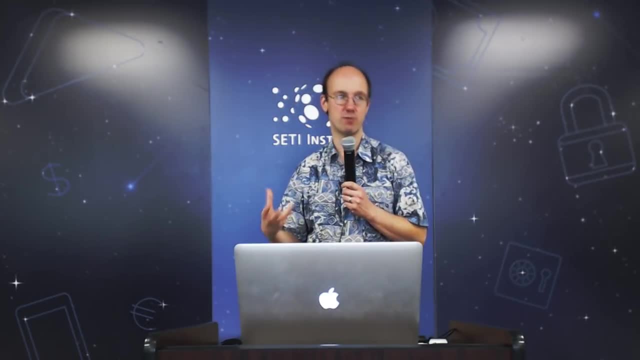 atmosphere is unpolarized or light that's scattered by the dust on the telescope is mostly unpolarized. Light that reflects off a planet might be polarized And if it is, that would help us pick that signal out. So if planets have significant polarization fractions, 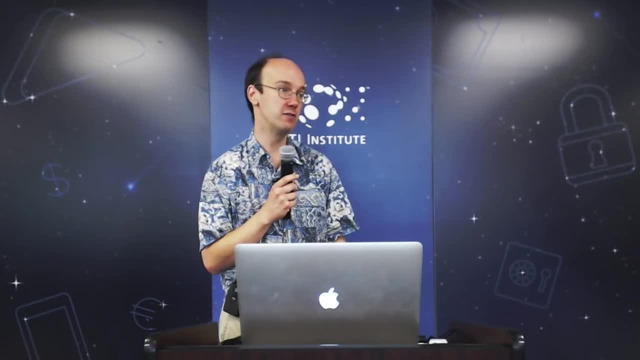 like 10% or 20%, then a one or two AU planet around maybe even four or five stars would be, would be within the detectable range if you spent persuaded the observatory to let you spend 10 or 20 or 30 hours on it. 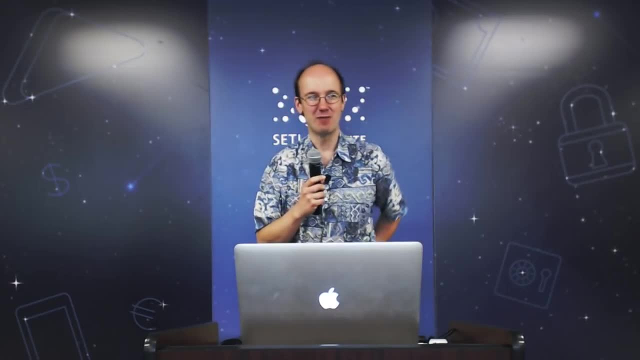 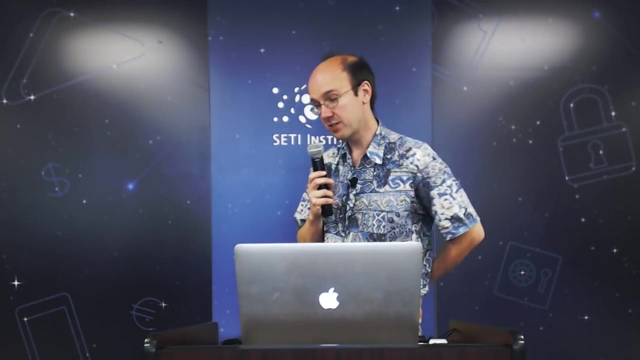 So I'll do epsilon or you can do alpha centauri- It would be a good combination. for it, There are models that predict the reflected light polarization. The Europeans are maybe looking for it, maybe not The self-luminous planets we talk about. 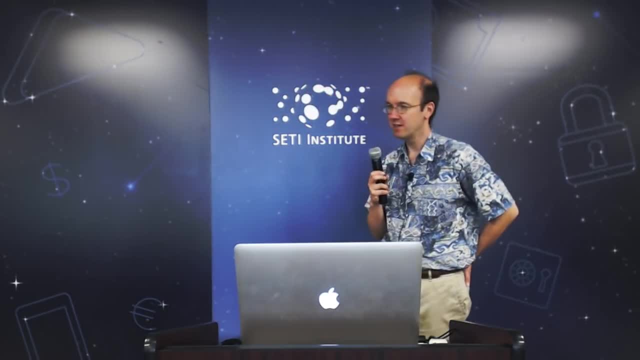 might also be polarized, but for reasons too complicated to go into right now. But GPI has shown to be very, very, very, very, very, very, very good at making those precise polarization measurements at the part in 1,000 level. 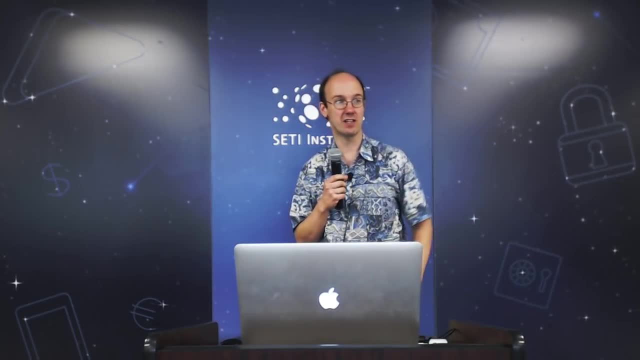 So our speckle suppression factor for polarized light might be 10 to the third, which does get us down, if we have enough photons, into the regime where we could hope to see these things. Can you tell us more about debris in 51 Eridani? 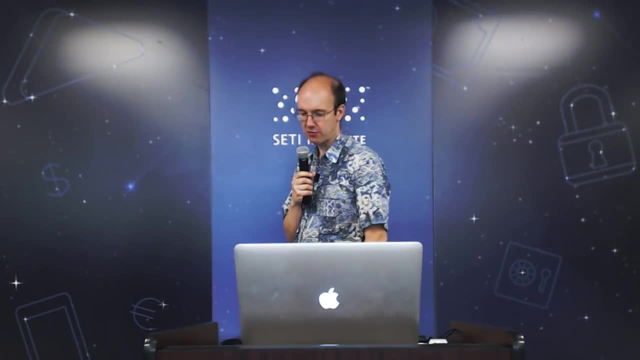 Is it imaged or is it just from the spectral distribution? It's just from the spectral energy distribution, So we can tell these debris disks, most often because the dust from the asteroids and comets colliding with each other absorbs visible light. It absorbs light. 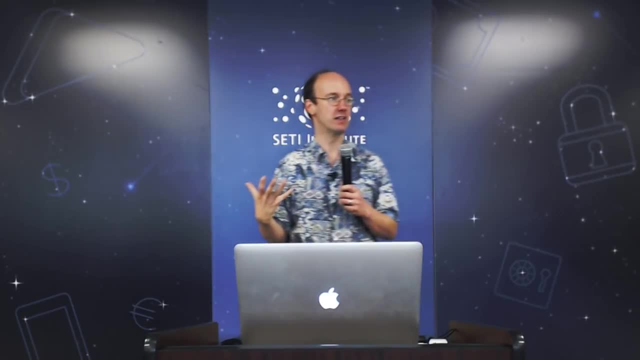 It absorbs light And radiates infrared light. So the signature is: you see extra infrared light from a lot of stars And you infer that that's from dust material or aliens, But dust is probably a more robust experience. in general, though, people talk about Dyson spheres and things like that. 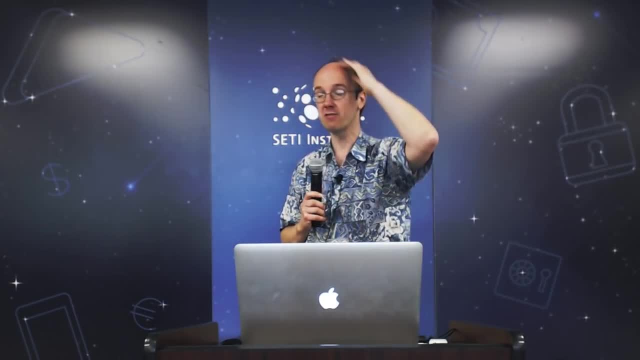 The 51 Erie case. its dust disk is actually pretty thin for such a young star. It's only about 10 times as much as the amount of dust in our solar system, which, for a 20 or 30 million year old star, is quite young. 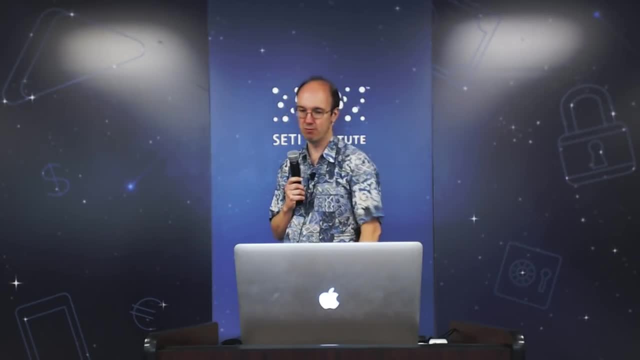 It's almost certainly undetectable, especially because the planet notionally clears a gap in it. Somebody, I'm sure, will be looking for it with a Hubble Space Telescope, which is very good at seeing dust at relatively wide orbits, But there's no detection yet. 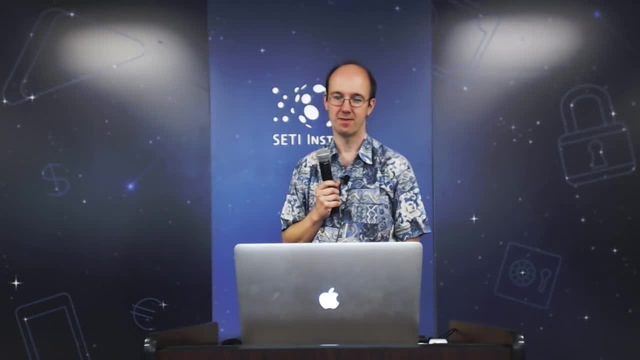 So I know with brown dwarfs you can see patchy clouds or some kind of cloud modulation as the planet rotates. Has the spectrum changed when you went back to look at it again, Or do you think it might Just got off the airplane a week ago? 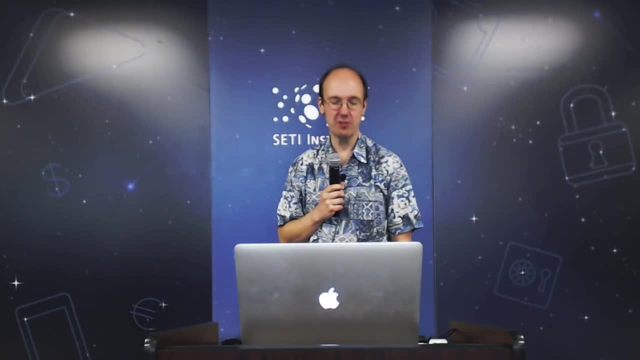 So ask me in a little bit- People certainly do think it might- for some classes of planets that you'd see the same kind of modulation as the clouds come in and out of field of view. It's a hard measurement. You could see how big the error bars are on that spectrum. 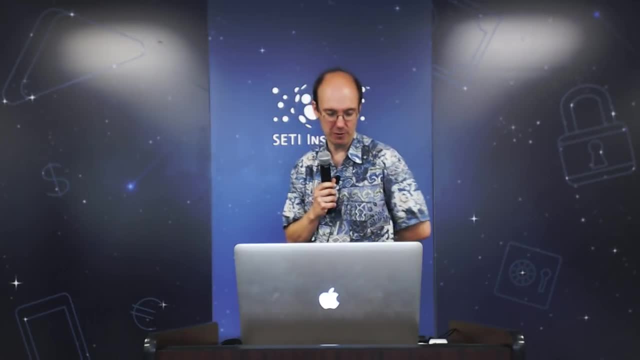 But it's certainly on our list is to try and monitor it And the trip I was on. I was in Chile for five nights And we only really had one good night, so can't tell yet, But I think it's unambiguously worth pursuing. 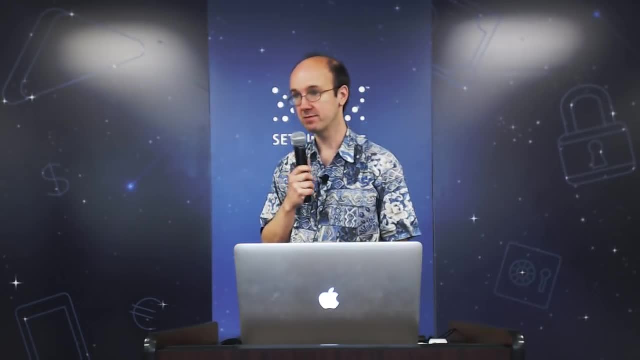 especially if it is at sort of 45 degree or more inclination. Bruce, great talk, Did you? did you mention that you've got future work? Are you queued up in slides that you could show us in a minute? I had a little bit about future space missions. 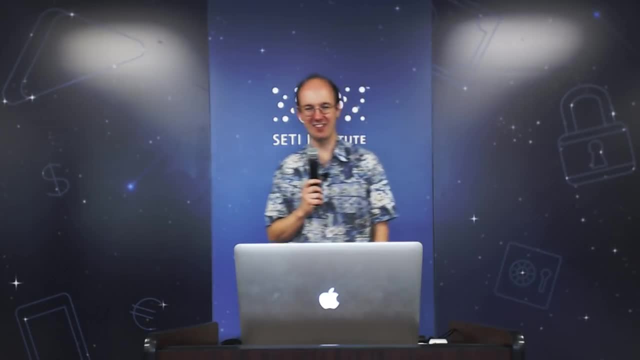 especially the W-first AFTA space mission. I wouldn't mind seeing a slide or two if we've got time. Well, we've got a couple of minutes And we're a little past the hour, but if nobody's flying up, People can leave too. 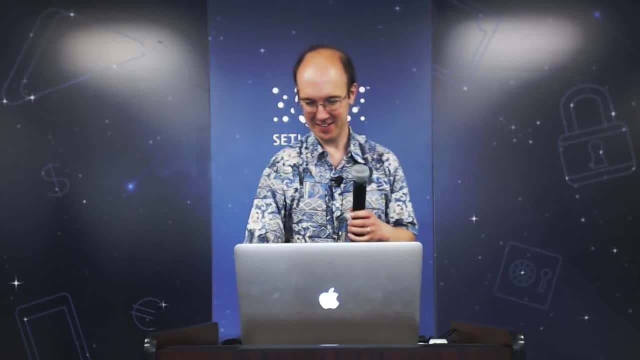 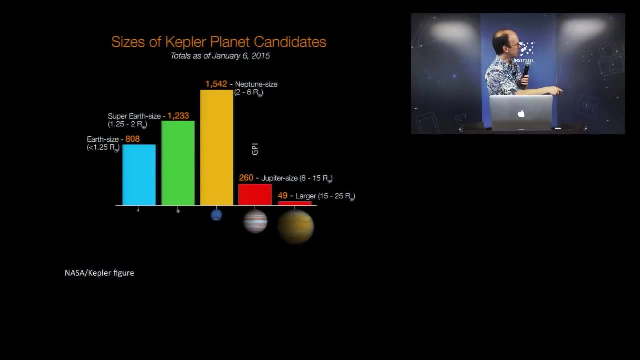 I assume they unlock the doors at this point. W-first, Yeah, W-first. Let me just do two or three slides, And I also had a little bit about the 30 meter telescope. So the broad question beyond is: GPI is really limited still. 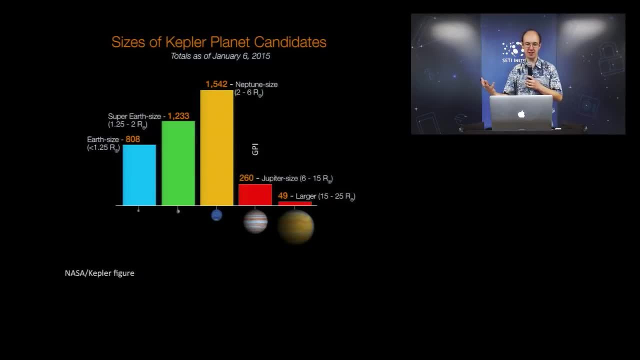 to these Jupiter size or bigger than Jupiter size planets. Kepler says that's not the most common kind of the planet in the universe. How are we going to characterize them? A lot of missions will do it, including the test mission, the sort of son of Kepler. 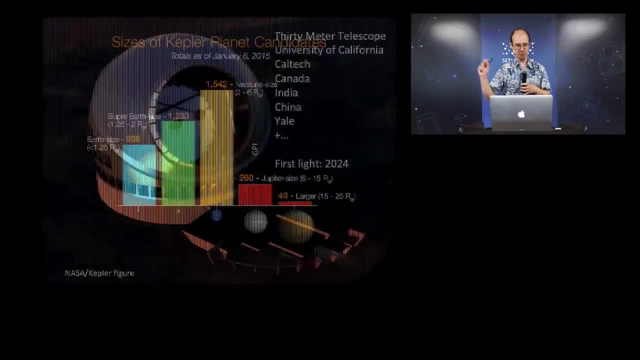 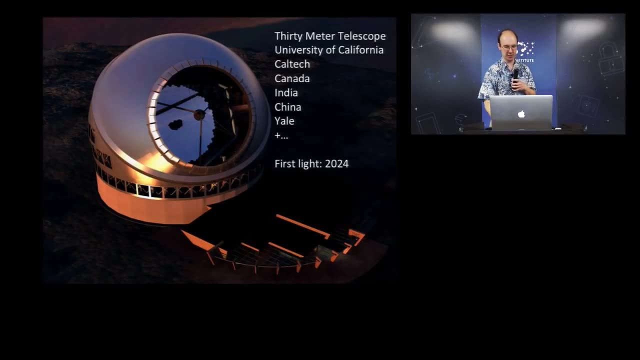 But ground-based imaging has a role to play too. The first way to do it is to put something like GPI on a really big telescope, like the proposed 30 meter telescope in Hawaii or its equivalents in Chile. That would probably get down to kind of Neptuny planets. 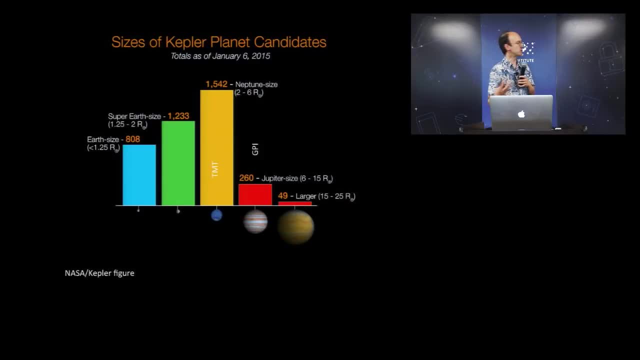 and scrape the super Earth regime. Another approach would be future space telescopes. Russ is involved in a proposal for one that would reach exquisite levels of sensitivity around very bright stars. so to probe Alpha Centauri, A broader version for slightly bigger planets. 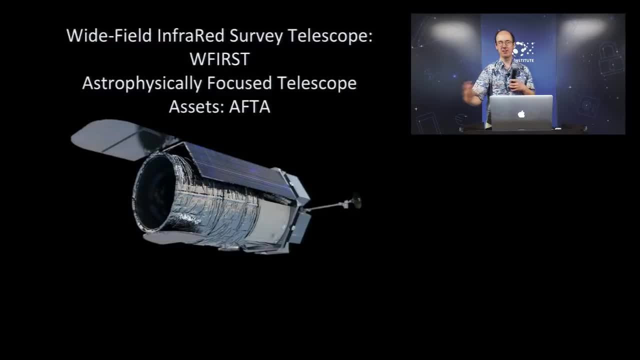 is something called W-first, So the acronym. it's going to get a real name when we fly it, But for now it's W-first Wide Field Infrared Survey Telescope. So the first part of its name tells you what it was originally intended to do. 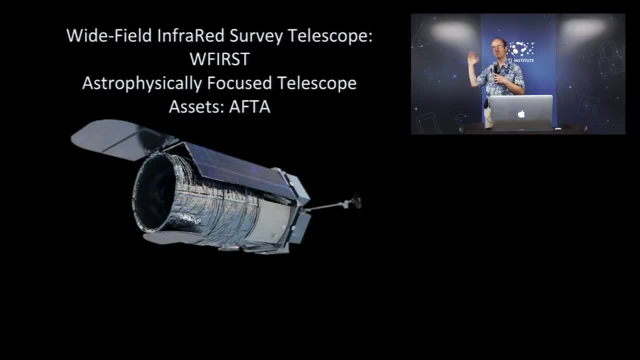 which is to survey the whole sky at infrared wavelengths for dark energy- cosmology stuff that a number of my colleagues find extremely. I'm being videotaped, aren't I Stuff? that a number of my colleagues find extremely exciting, And so it was proposed and ratified. 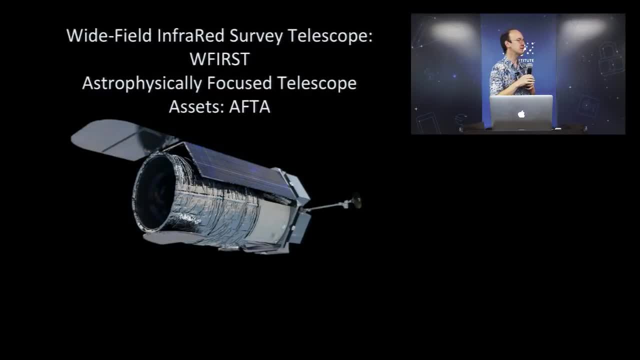 by the sort of astronomical community as the most important thing we could do in the next decade. It was originally going to be a, so the second part of the name, Astrophysically Focused Telescope Assets. That's even worse than Wide Field IR Survey Telescope. 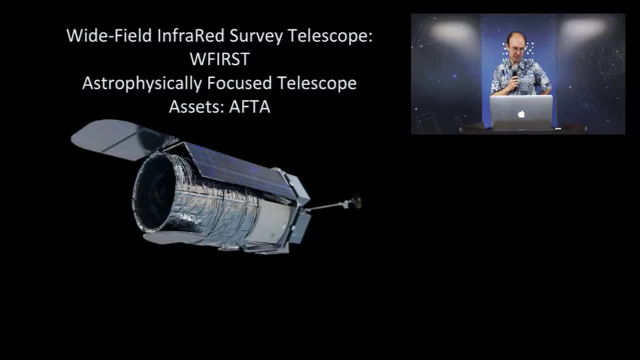 because it's not a word. Where does that come from? So W-first was originally going to be about a 1.2 meter sort of Kepler-sized telescope, extremely wide field of view, infrared camera, and it would basically do counting galaxies and measuring their shapes. 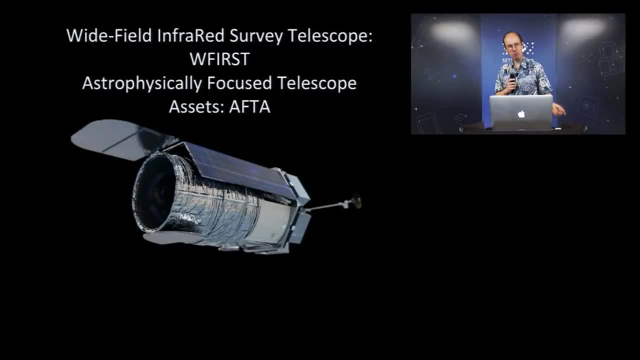 Over a three to five year mission. it could only do that. Then something weird happened. So the way I explain this is: let's say you like hiking a lot, You might buy hiking boots and they might be on sale, So you might buy a bunch of hiking boots. 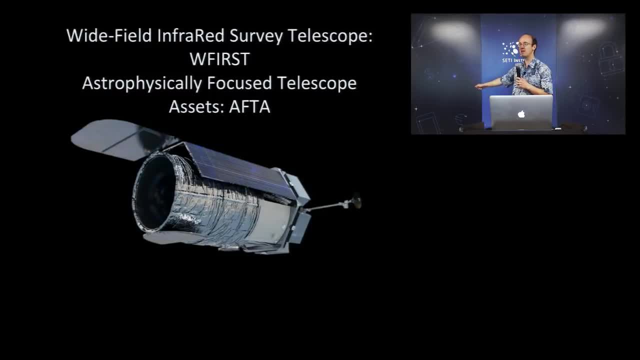 Then you might forget you have them. Then you open your closet and you discover you've got eight pairs of hiking boots- Clearly too many. You have some friends, so you say: would you like some of my hiking boots? You donate them to them. 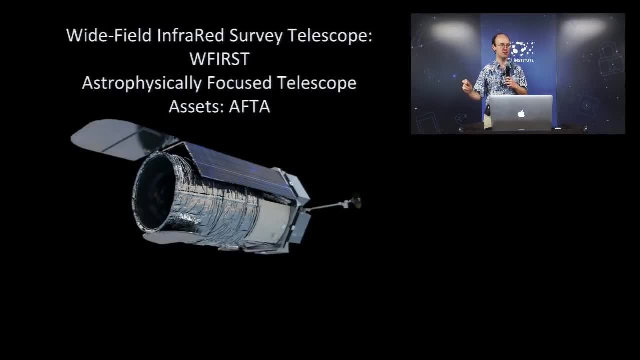 The same thing happened with the Department of Defense and NASA, Except, instead of hiking boots, you should think, Hubble Space Telescope-sized telescopes. So the Department of Defense opened their closet and they discovered- I do not know how many they have, but they definitely had too many Hubble Space Telescope-sized 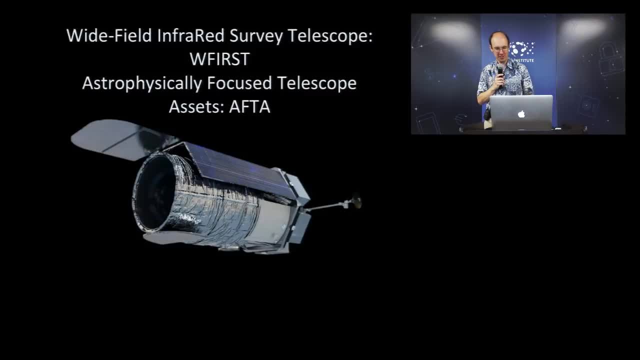 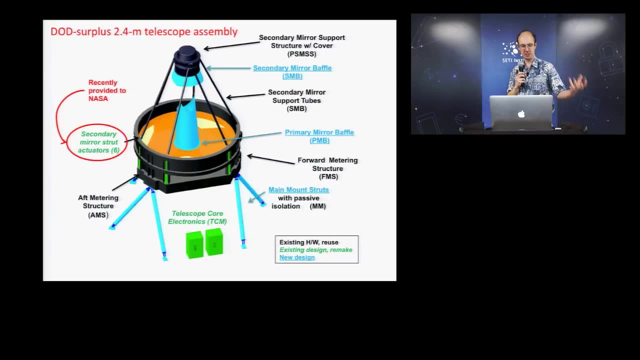 telescope assemblies hanging on a hook somewhere, And they donated two of these to NASA. So 2.4 meter telescope assemblies- not whole spacecraft, just the telescope and the optics, but designed for a wide field of view, So great for the dark energy science. 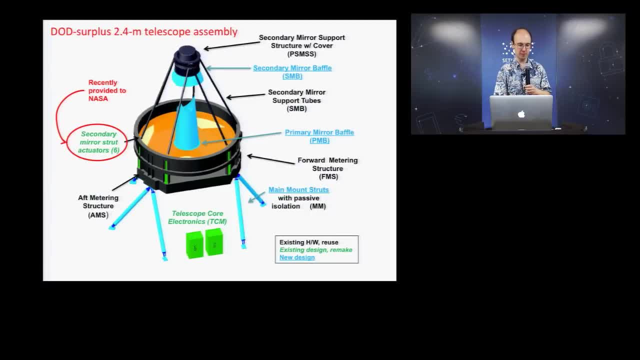 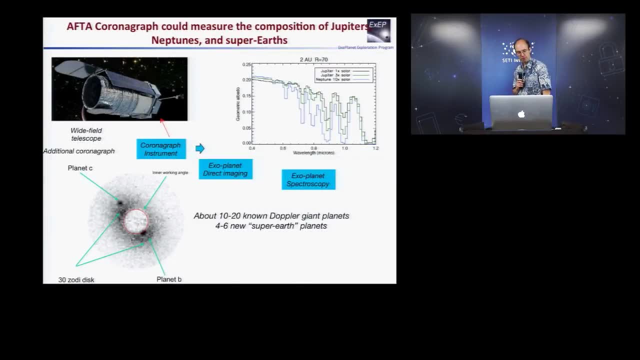 Big, optically good, robust and available, And if you're going to do that, I'll skip this animation, Although it's very cool. There are a couple of good things: 2.4 meters. first of all, it's big enough. 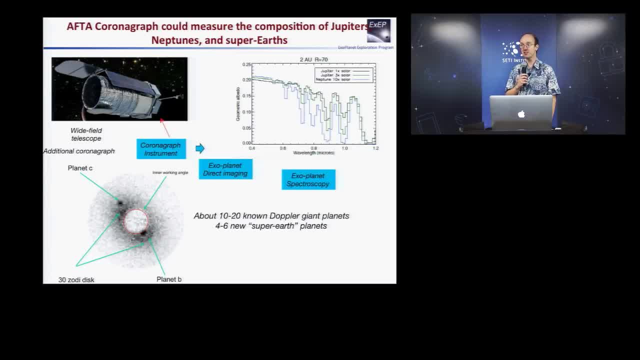 that it can do the extremely exciting galaxy counting stuff much faster, so it doesn't take all five years of the five-year mission, which gives you some time to do other stuff, like, say, look at planets, And it's big enough that you could actually use it. 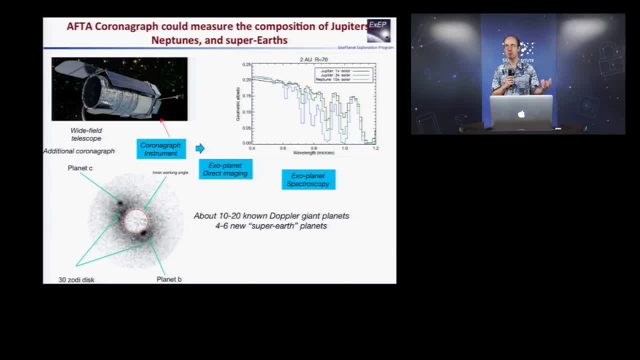 to do direct imaging of exoplanets, which is hard to do on a one-meter telescope but very practical on a 2.4-meter telescope. So the baseline is to add something, basically, that looks like GPI, a deformable mirror, a coronagraph mask. 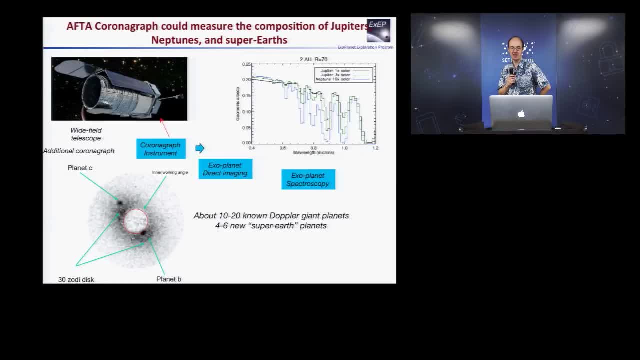 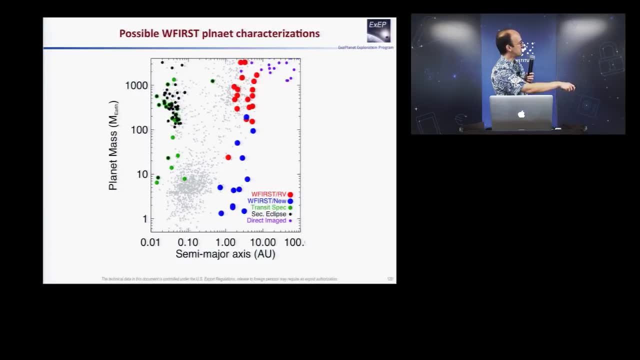 to block starlight, an integral field spectrograph, And fly it on this and do characterization of extrasolar planets in reflected light And in the usual mass semi-major axis diagram space. from some simulations Dmitri Sivransky at Cornell did it could reach down to maybe even Earth-mass planets. but definitely to the sort of super-Earth planets several times the mass of the Earth, and expect to discover, get photometry, maybe spectra, maybe not, but definitely characterization of a decent sample of those, if it flies, which it has a good chance of doing. 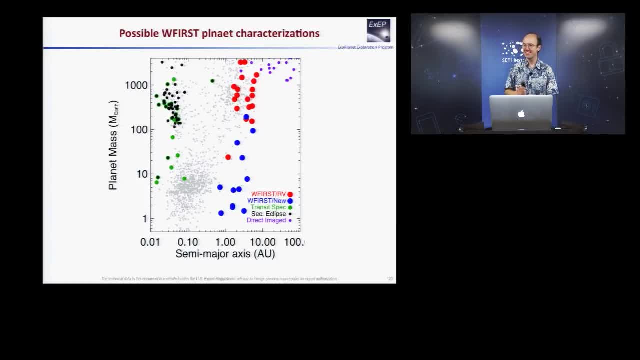 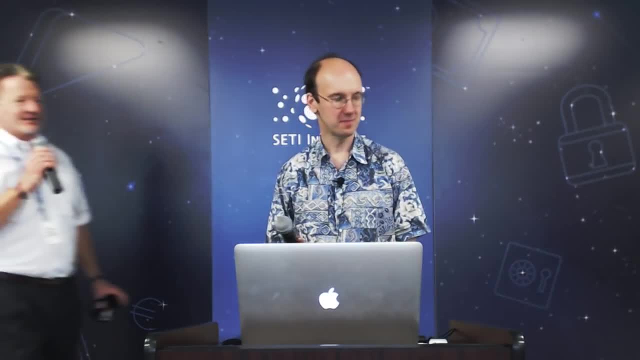 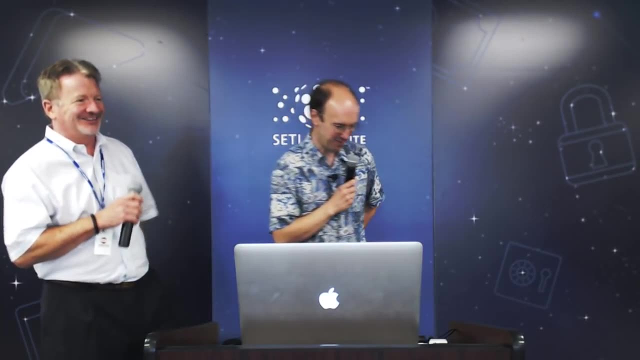 And that's the W for 2024 or so. So that's the W for sideline. Well, if there's no other questions I would like to do you want one last quick one, Excellent question. So if you were to, no atmospheric turbulence. 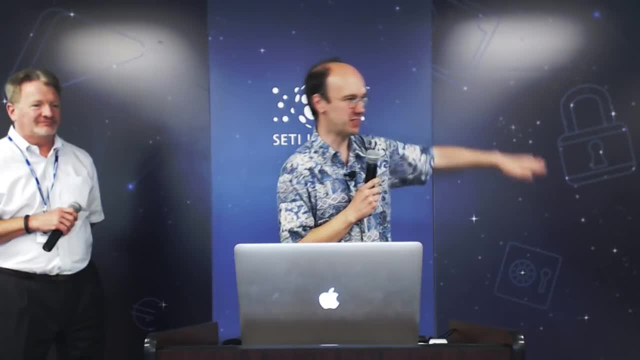 but there's still imperfections. in the mirror of the telescope It's better than the Hubble mirror. It doesn't have the big misspheric elaboration in it, But just the act of polishing it puts tiny little ripples in the mirror from the tools. 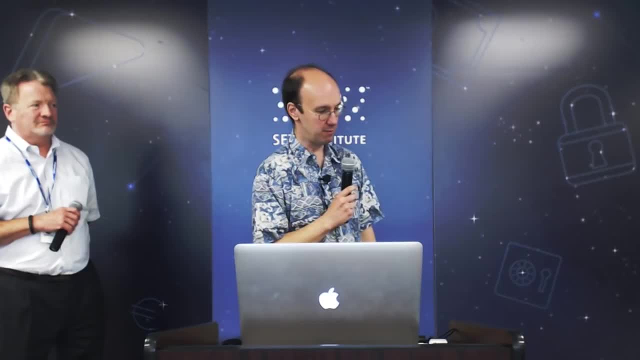 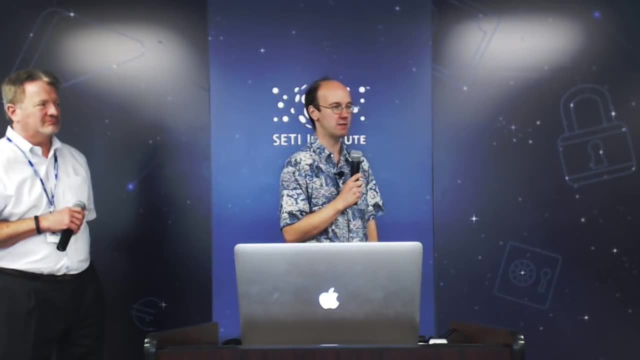 you use to polish it. To actually see a planet without any correction, the size of those tiny little ripples would have to be smaller than an atom. They would have to be a tiny fraction of an angstrom or a nanometer. You can't make a mirror that precise. 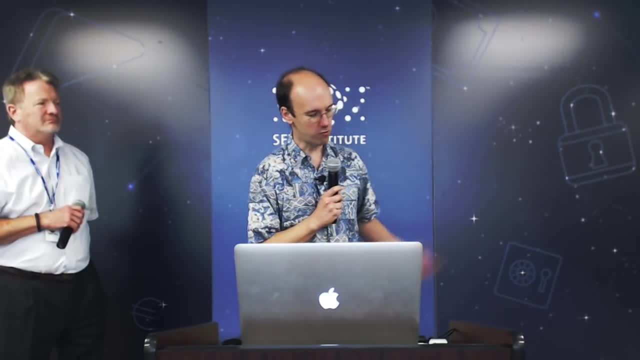 and you can't count on it staying that precise as you fly it in space. So the deferral mirror cancels the aberrations intrinsic to the optics as well as more complicated diffraction. Russ is wincing, because I'm oversimplifying this. 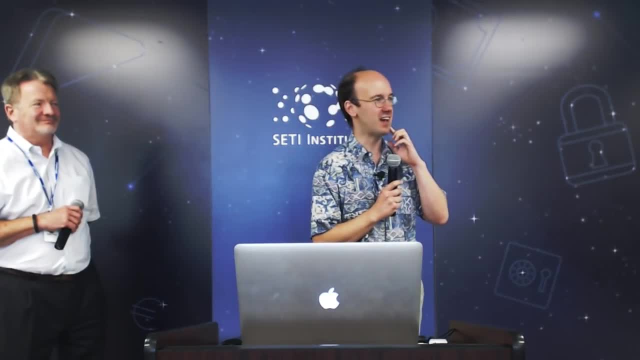 But as well as more complicated optical effects intrinsic to the design. So it's to fix the little polishing errors and imperfections. That's why you can't do this with Hubble, but you couldn't do this with any space telescope. It's much easier to build it properly, much easier. 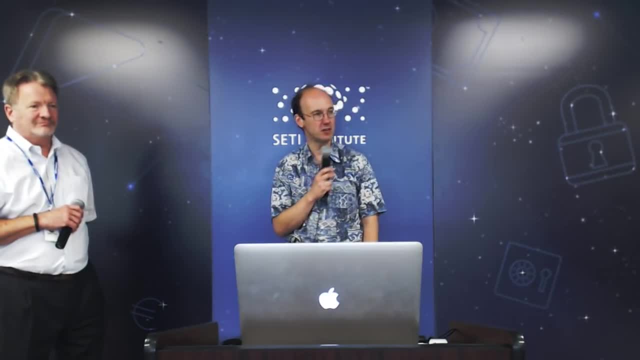 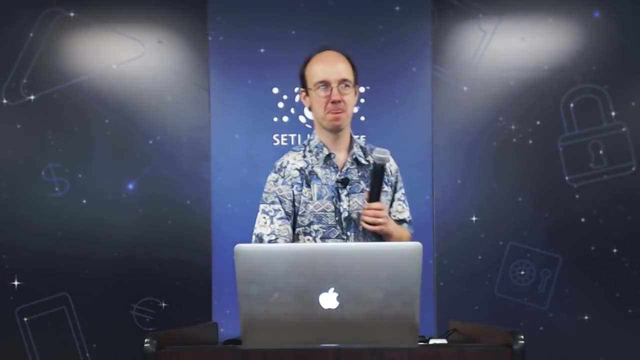 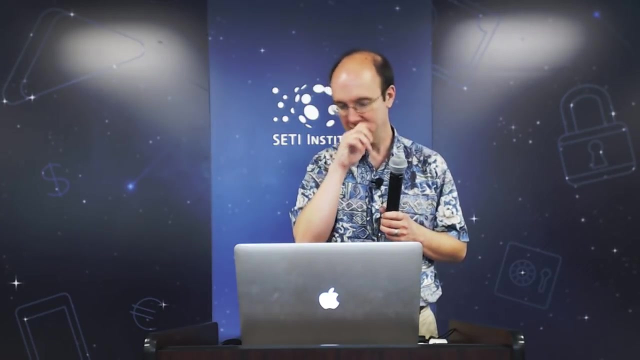 to correct it rather than to try and polish it at that sub-ultra-mega-nanometer level. OK, One last question I was wondering: with GPI or maybe future surveys like this, is it at all possible or likely that we could get a long enough time?